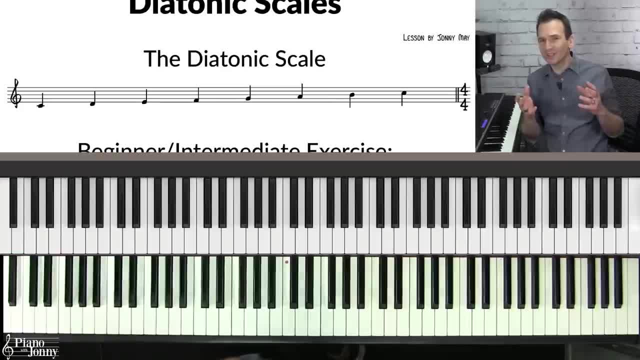 specific way, which I'm going to talk about in just a minute. you're not really going to understand how to use major scales in jazz, So I'm going to walk you through this exercise. I'm going to start with the beginner version, then intermediate and then advanced Okay. so if you're a beginner jazz, 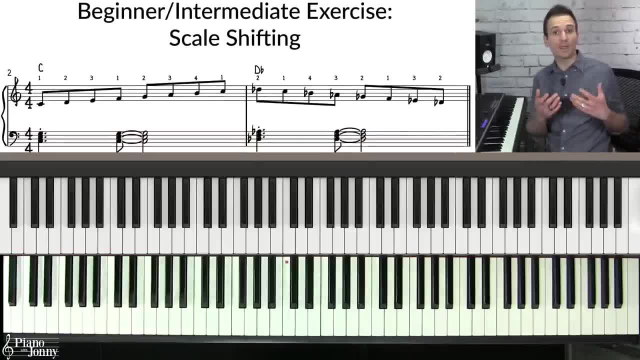 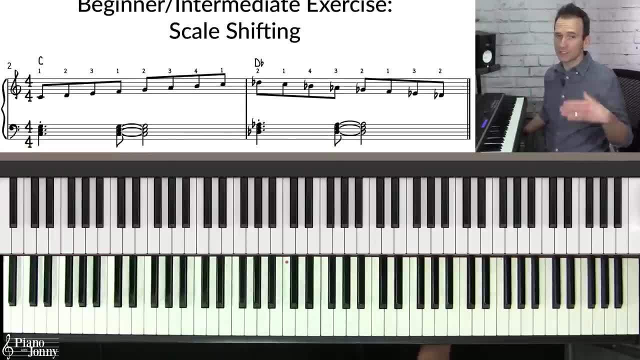 pianist, how do you play your major scale? You might be thinking: well, how do you play your major scale? How do you practice your diatonic scale or major scale, so that you can successfully improvise jazz piano? Well, first of all, you need to know your major scale in all 12 keys. 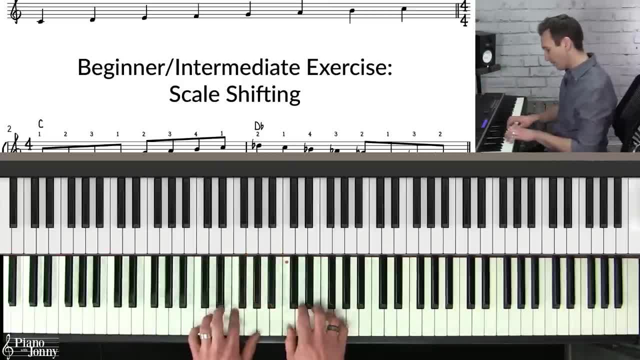 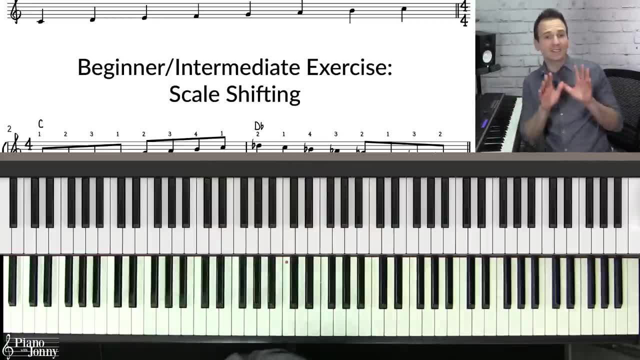 But I do not recommend that you practice your major scales by playing a scale up the piano and then doing it in the key of D flat, like so many students practice them Instead. what you want to practice is called scale shifting, And this is when you transition from one major scale to another major scale very smoothly. 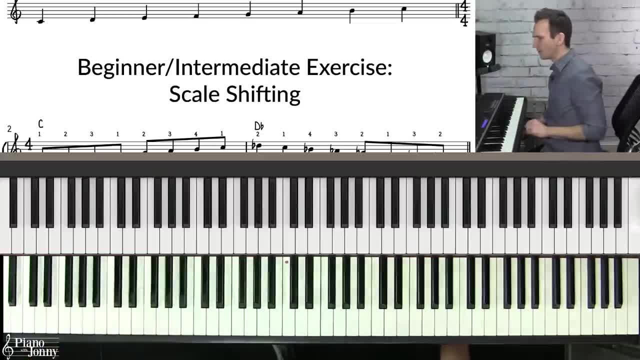 And this is a hallmark of jazz playing. So let me show you what I mean. I'm going to briefly solo on all the things you are and I'm going to show you what it sounds like to smoothly transition between two major scales: A flat major and C major. 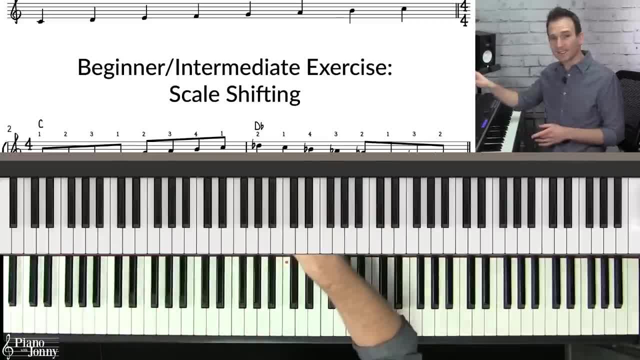 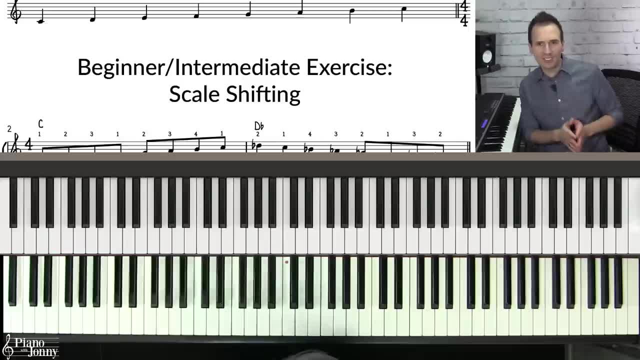 How was I able to do that? Well, it's through practicing the exercise that I'm about to show you. But before we do that, if you're enjoying this lesson, please hit the like button, And if you're new to the channel, be sure to subscribe for more videos just like this. 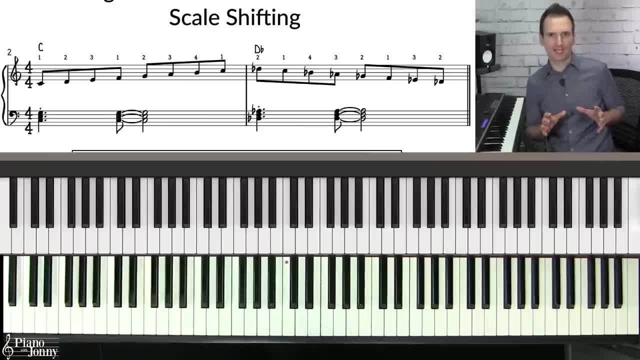 What you want to practice is called the scale shifting exercise, And with this exercise you end up practicing all 12 of your major scales, But, more importantly, you practice transitioning between the scales so that you can get some really nice smooth lines. So here's how it works. It's actually really simple. 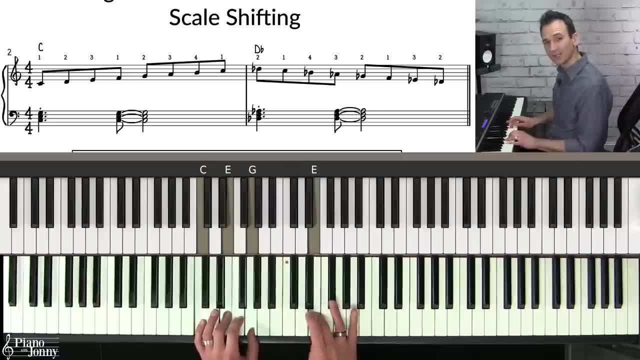 We're going to play the C major, scale up the piano. We're going to use the standard fingering for C. Okay, so thumb under. And when you get to the high note C, we're going to use our thumb. And guess what we're going to do here? 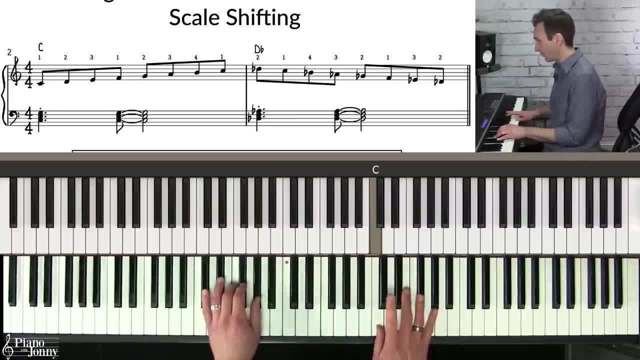 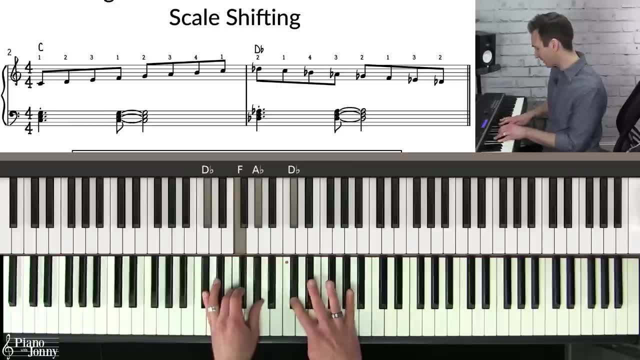 We're going to transition to the D flat major scale coming down, but we're starting on our two finger, So we have You see that. So what I did is I'm playing my D flat major scale. I'm starting on the two finger. 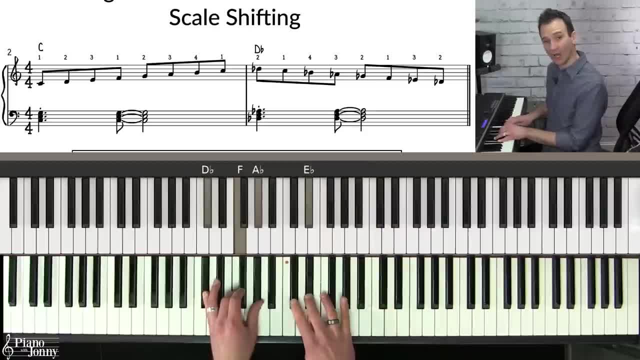 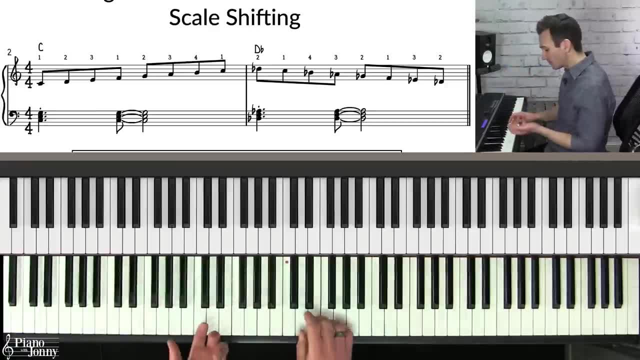 Crossing finger four And playing the standard fingering on D flat. okay, And once again, it's not just about practicing your major scales, It's about transitioning between them smoothly. See what's happening. And so this is kind of the first step of building jazz lines. 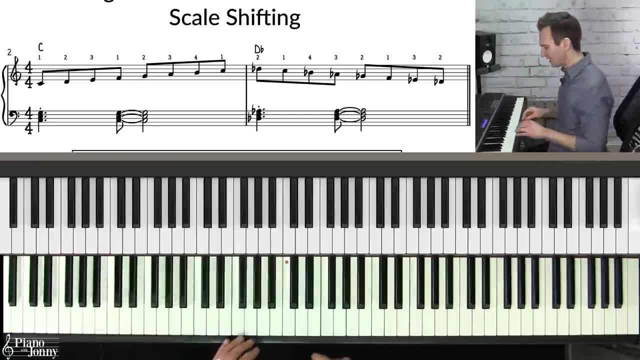 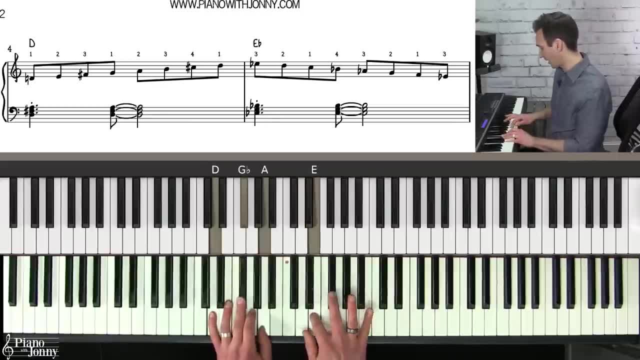 You have to be able to switch between scales in a smooth manner. Okay, so we left off on the D flat. Let's go to D major. That's going to be the thumb. We're going to play this up: Standard fingering. 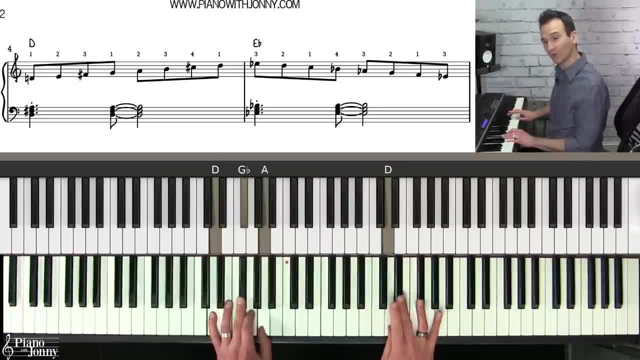 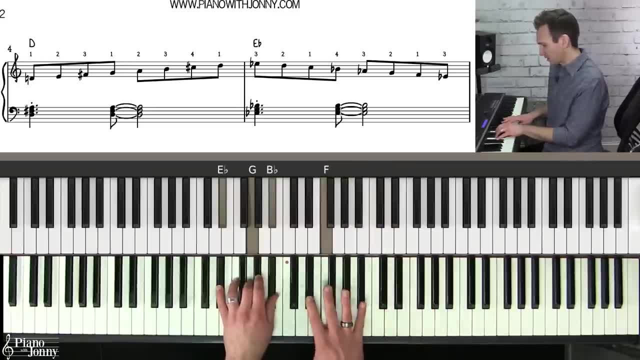 And then, when we get to the D, guess what we're going to do on the E flat. We're going to use that third finger And we come down on E flat. Okay, You see what's happening. So we're very quickly shifting between scales. 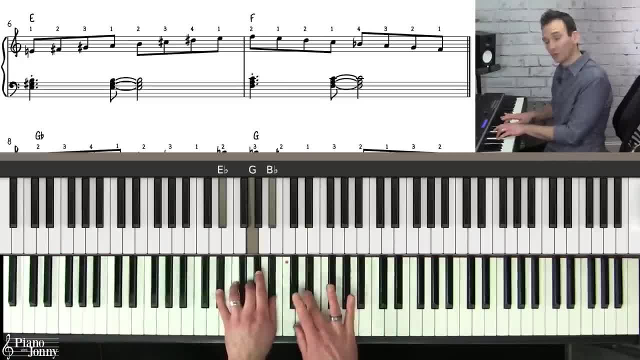 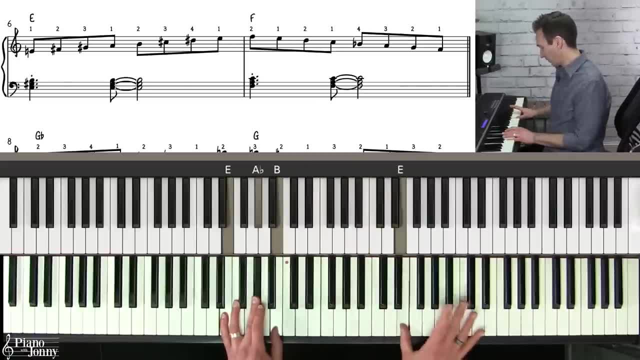 Okay, so once you land on E flat, By the way, you can use the two or the third finger there. Then we go to E. That's going to be the thumb Standard fingering. We're going to use thumb there. 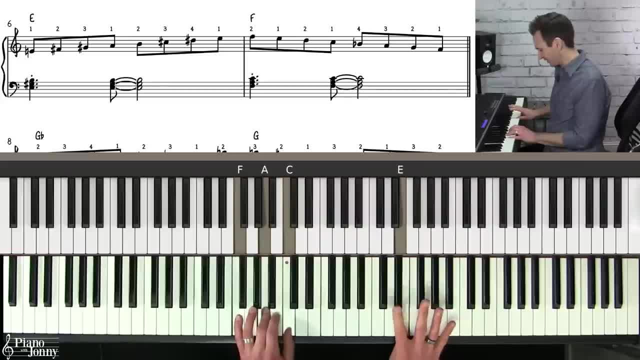 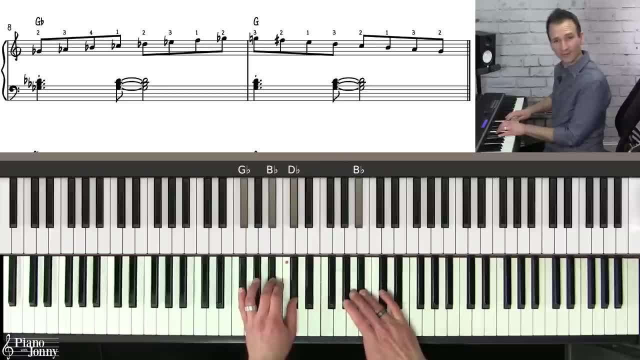 And then on the F, we're going to go two, Let's go two more, Let's go two, one, Four, three, two, one, Okay, And then G, flat two finger, Standard fingering. And then for the G, we're going to use that third finger. 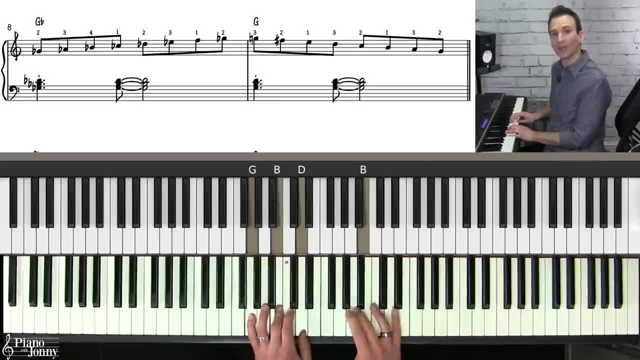 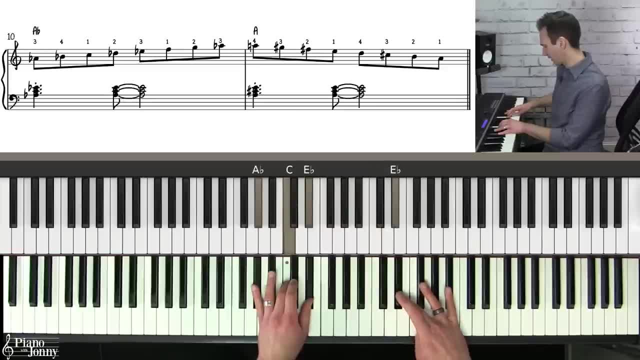 And we're going to go three, two, one, Three, two, one, three, two And then A flat third finger, And then we're going to go thumb, Standard fingering, Thumb, And then on the A we're going to use the four finger. 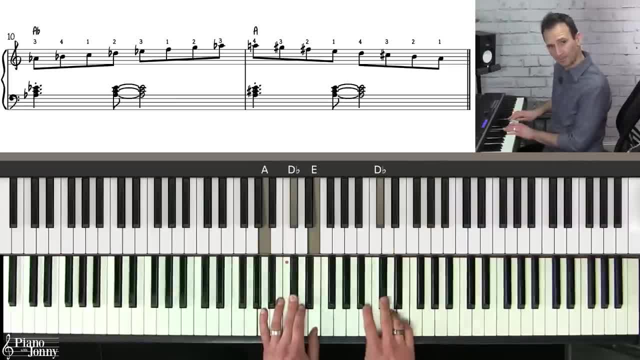 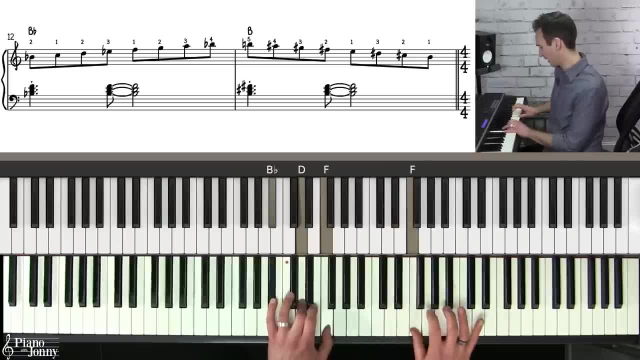 See what's happening. And then fourth finger on the D, And then finally B, flat second finger, We're going to come up with thumb, Third finger, And then for the B, we're going to use the pinky. It's going to be there. 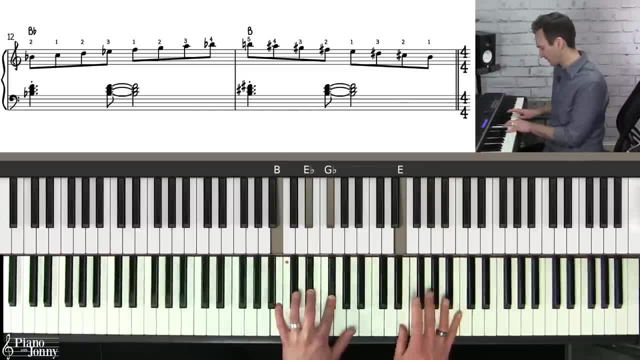 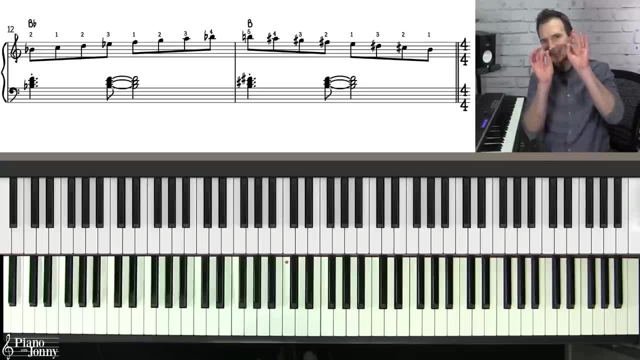 And we're going to take the scale down. This is the B flat major scale And end on the B. So what you just did is you practiced all 12 of your major scales, but you practiced that smooth transition between the scales. So if you speed it up just a little bit, 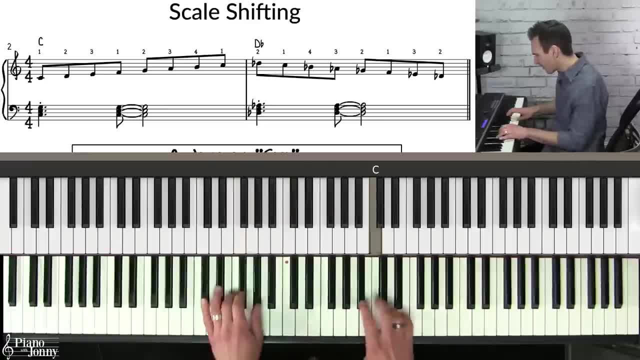 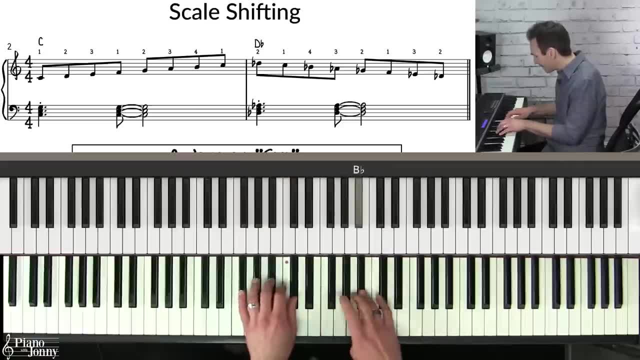 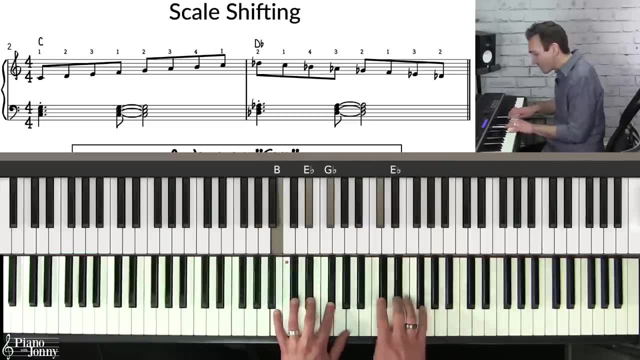 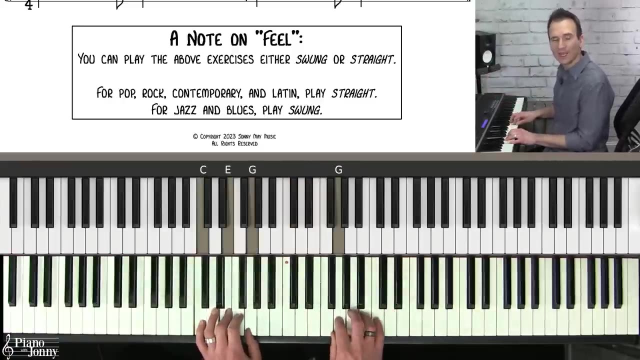 check out what it now sounds like. Now a quick note. You can swing your eighth notes like the way I'm playing it: One and two and three and four, and. Or you can play them straight: One and two and three and four, and. 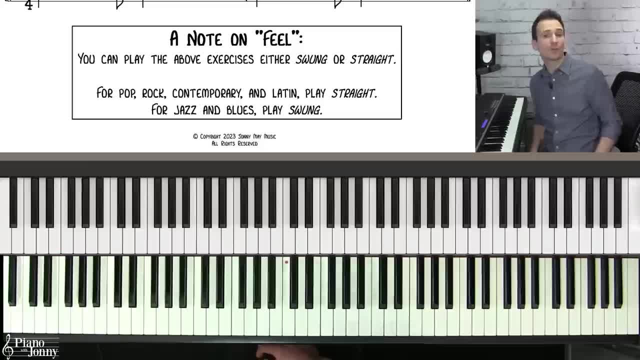 It depends on the style that you want to play. So if you're playing pop, rock, contemporary or Latin, you'll typically play your eighth notes straight, But if you're playing jazz or blues, you'll typically play them swung. Now, the goal tempo for this will be 100 if you're more on the beginner side. 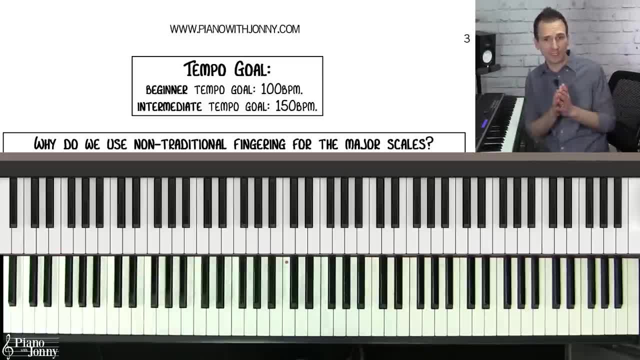 and it will be 150 if you're more on the intermediate side. Now, this lesson comes with two backing tracks for this exercise: one at the beginner speed, one at the intermediate speed. So let's go ahead and play this at the beginner speed. 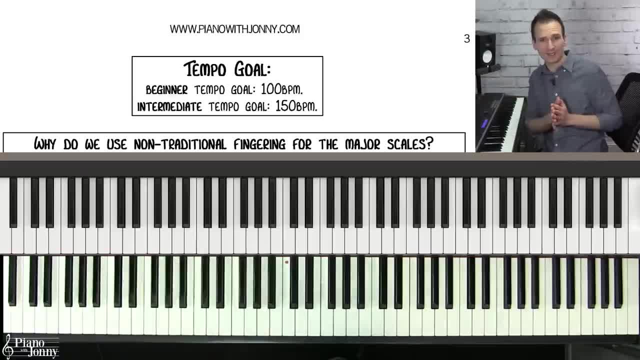 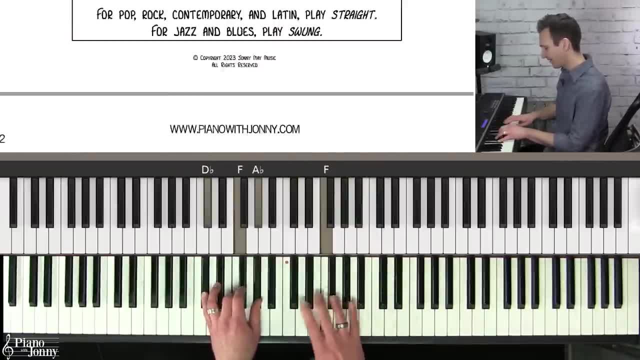 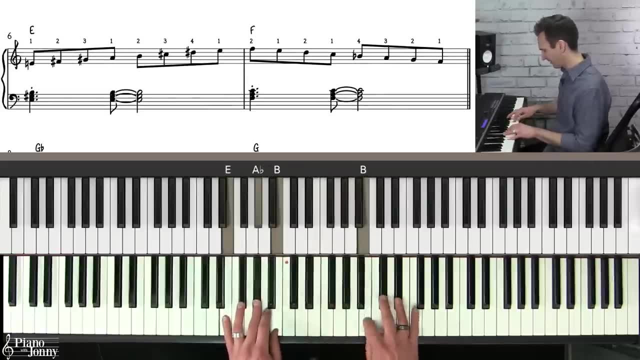 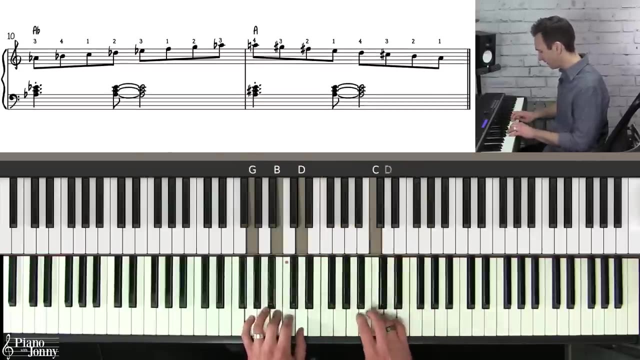 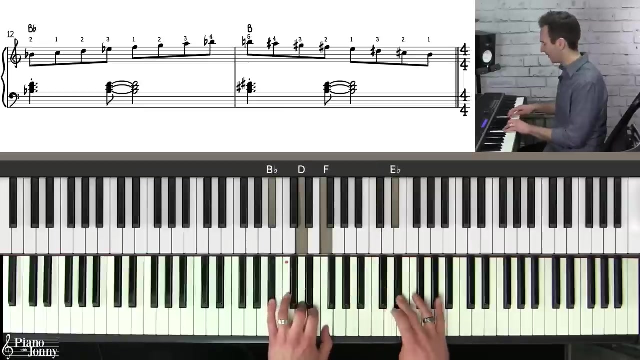 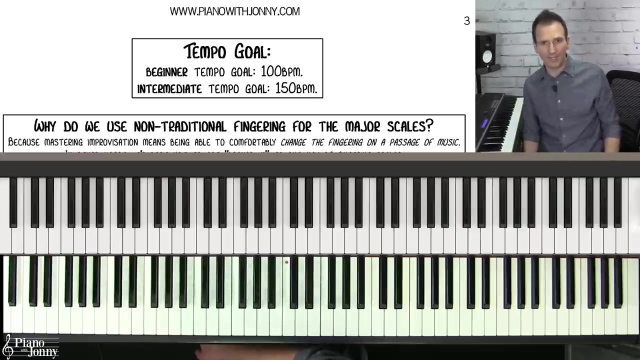 and then I'm going to teach you the intermediate to advanced level exercise. Here we go: D flat D, E, flat E, F, G, flat G A, flat A, B, flat B. By the way, this lesson comes with 12 downloadable backing tracks. 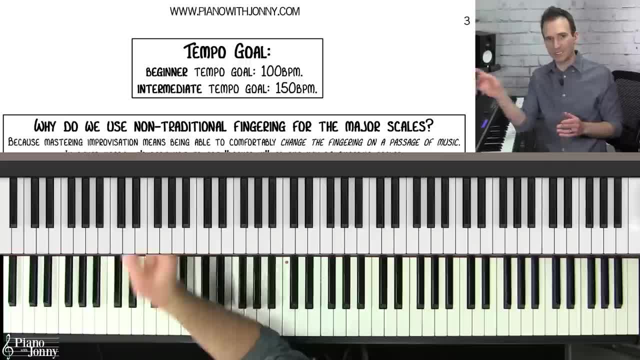 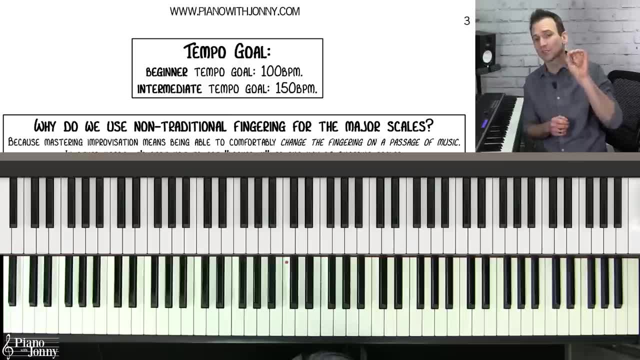 at different tempos. You can also download the lesson sheet music you're seeing on the top left of your screen and you can change the key of this entire lesson with the click of one button with our smart sheet music. So I'll put a link to all of that below. 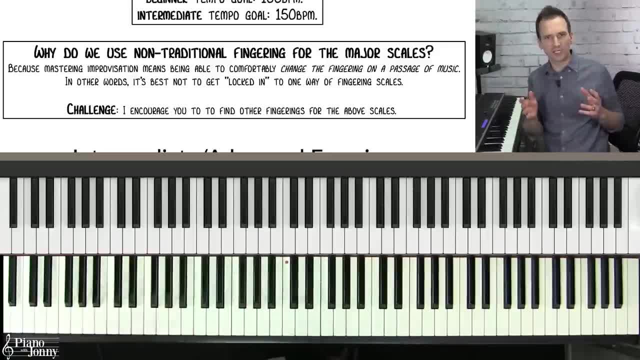 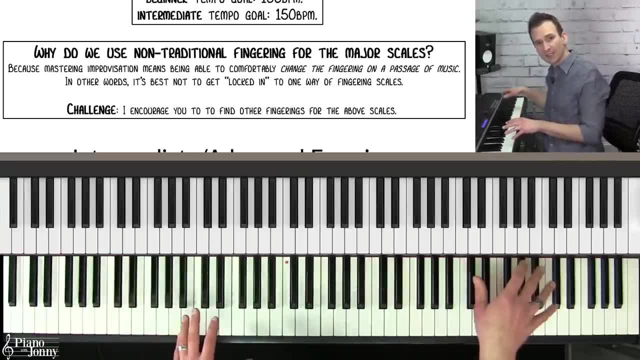 Now you may have noticed that the fingering of these scales is not traditional meaning. if you took classical piano lessons, this is probably not the fingering that you learned for each of these major scales. So why are we using this non-traditional fingering? 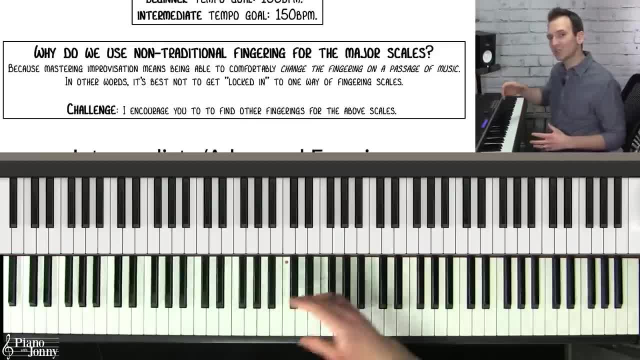 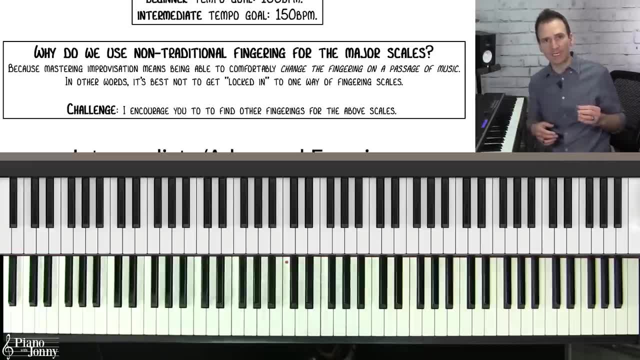 Well, whenever you're improvising at the piano, you want to be able to change the fingering on the scales that you're playing, depending on whatever type of passage that you're improvising, meaning that you do not want to get locked in to one way of fingering the major scale. 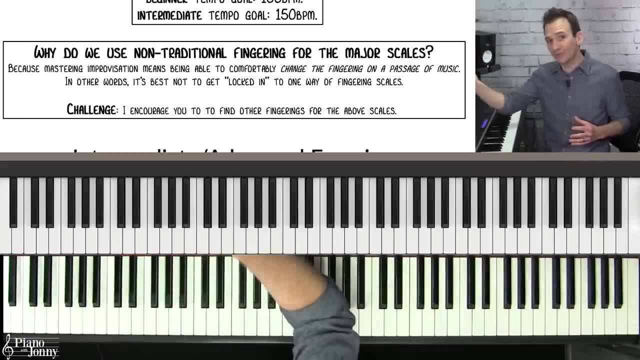 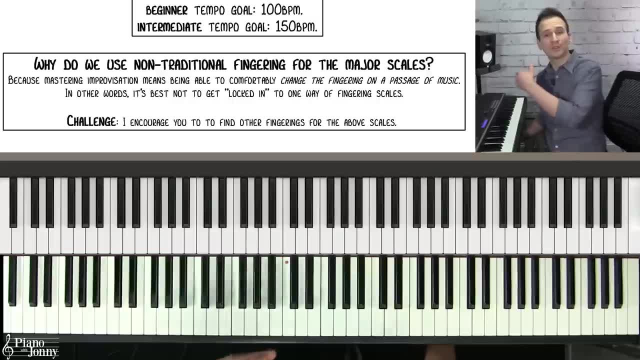 So something that I would encourage you to do is to actually come up with your own fingering for this exercise that you just learned. By the way, if you want to learn all 12 of your major scales, you want to learn all of your diatonic chords. 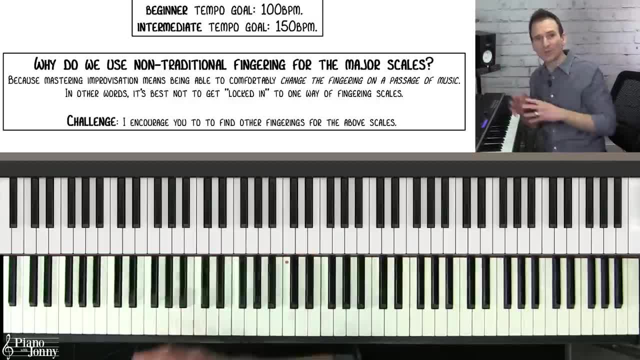 common chord progressions. how to play lead sheets with these chords accompany with them, you can in our Beginner Foundations Learning Tracks. I'll put a link to those below. All right, if you're more on the intermediate to advanced level, you need to know all 12 of your major scales to play jazz. 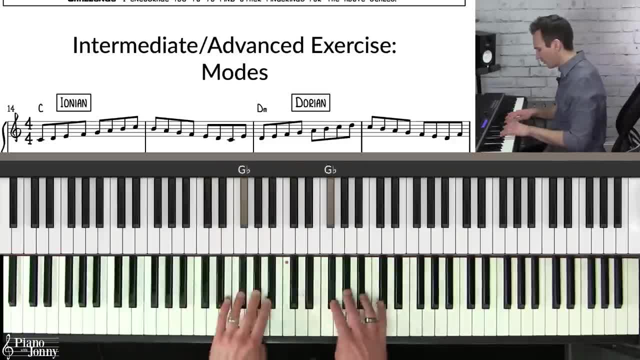 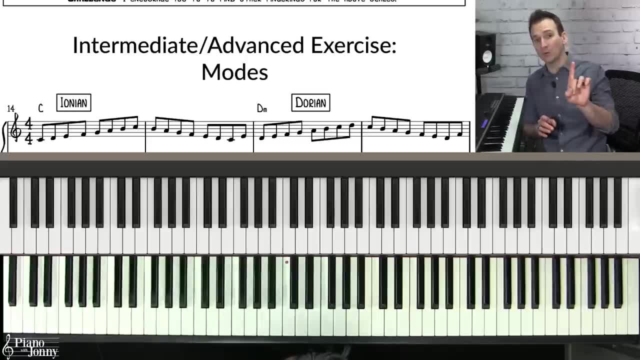 But again, I do not recommend that you just play your major scales up and down the piano. Instead, the best way to practice your major scales is to practice them as modes, And the modes are basically when you take the major scale and you start on a different note from that scale. 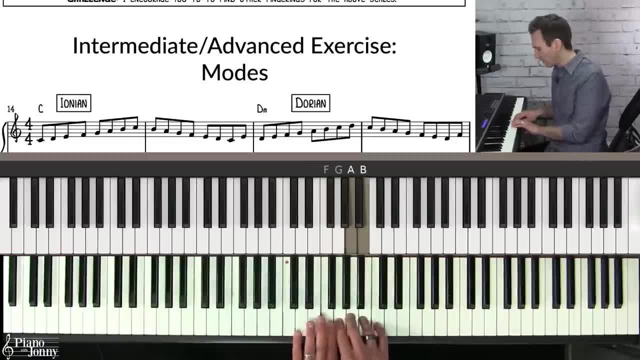 So if you play a C major scale starting on C, we call that Ionian. If you play the C major scale starting on D, we call that Dorian. This is called E, Phrygian, F, Lydian, G, Mixolydian. 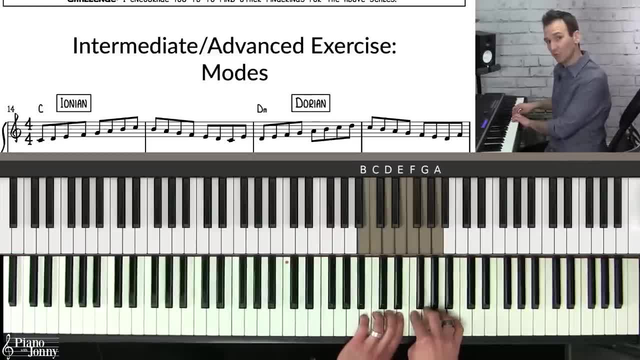 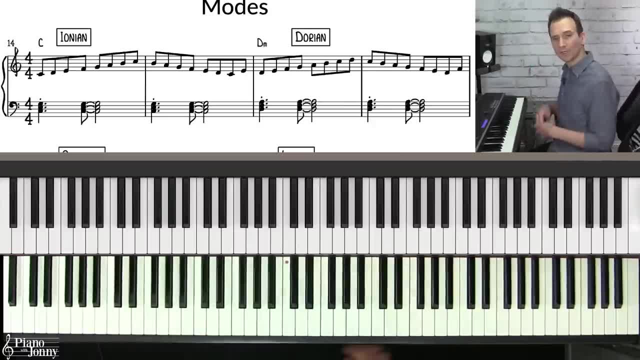 A Aeolian and B Locrian, And there are many ways to practice your modes, but one of the best exercises is this one. What we're going to do is we're going to play the C major, scale up the piano, We're going to bring it down. 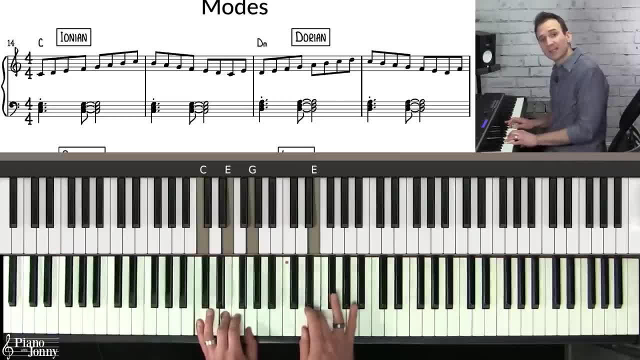 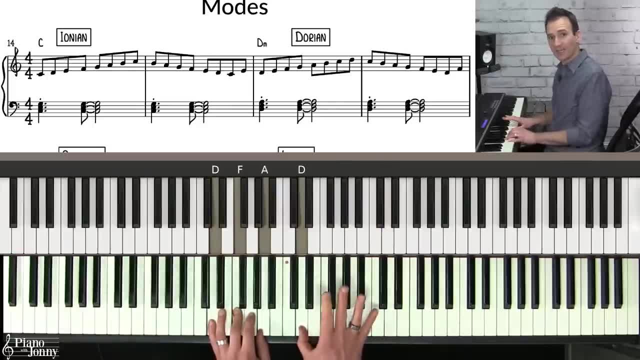 and we're going to do a little skip up to the E and this sets us up for D. Dorian, You see what we're doing. So it's the C, major scale, same fingering, except now we're starting on the D. 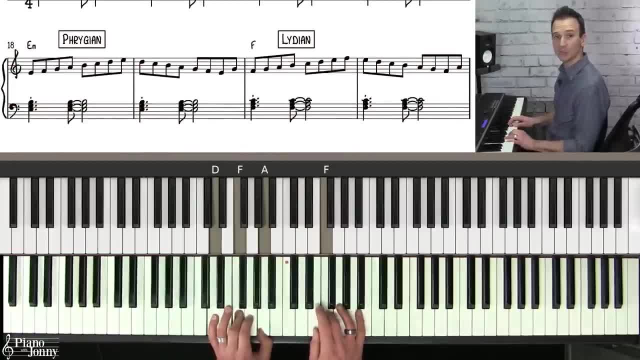 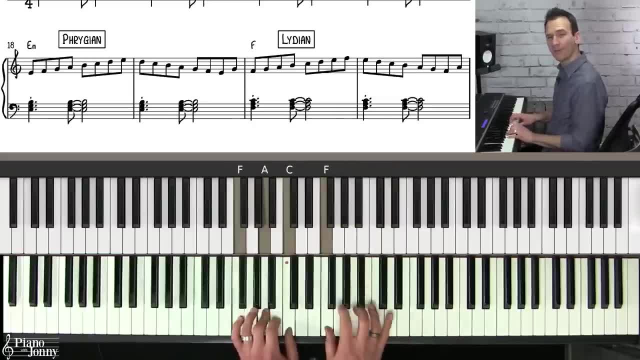 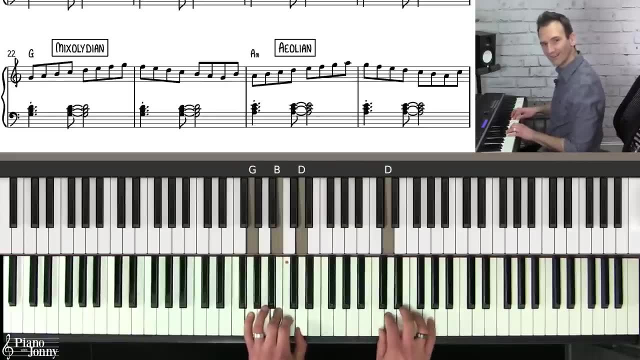 Now, from here, we use the transition note F and this takes us to E- Phrygian. See what we're doing. There's the skip to F, same fingering as the C. major scale. G, Mixolydian, same pattern. 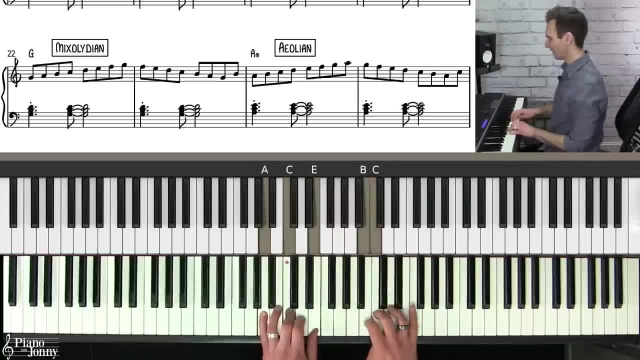 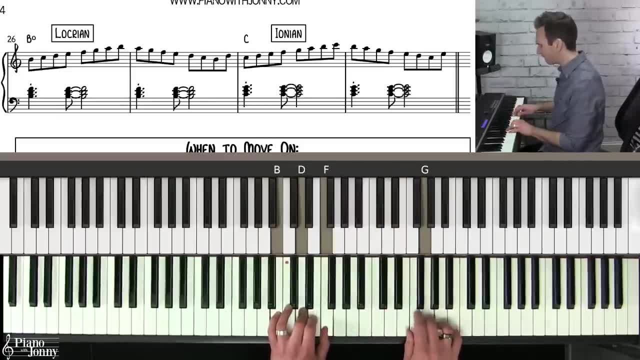 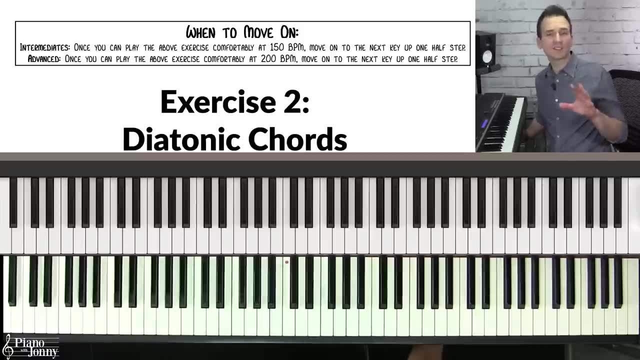 there's the skip now to A, Aeolian, B, Locrian and C. So the goal is to get this to a faster tempo. If you're more on the intermediate side, I recommend 150 BPM, and if you're more on the advanced side, 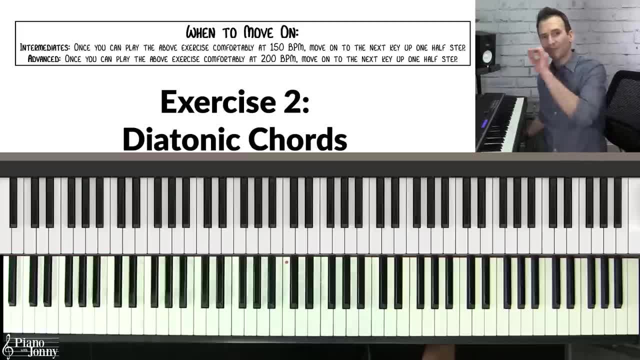 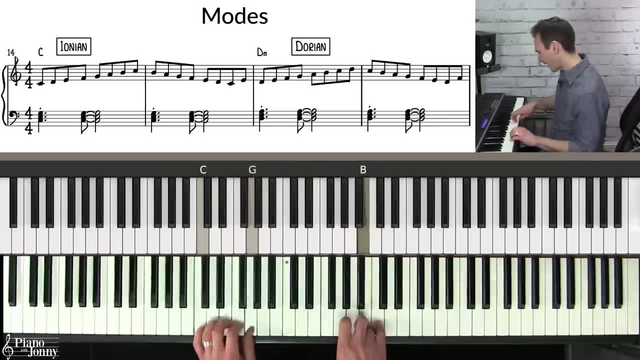 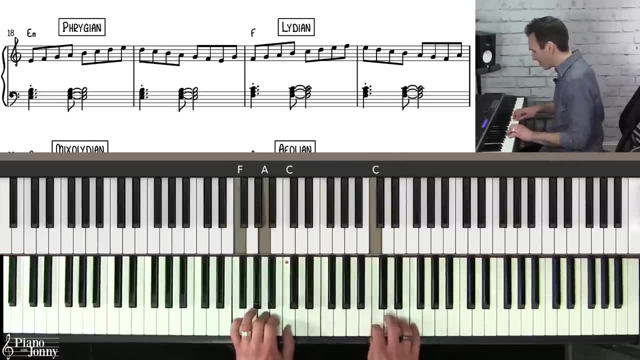 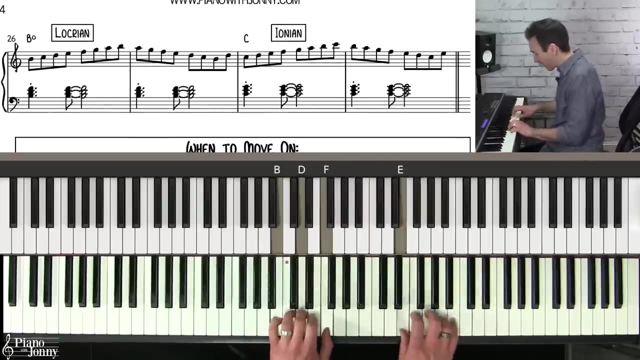 I recommend 200 BPM. So let's go ahead and play this with the advanced backing track at 200 BPM so you can hear what it sounds like. and here it is, Here we go, And once you're able to play, at the goal tempo. 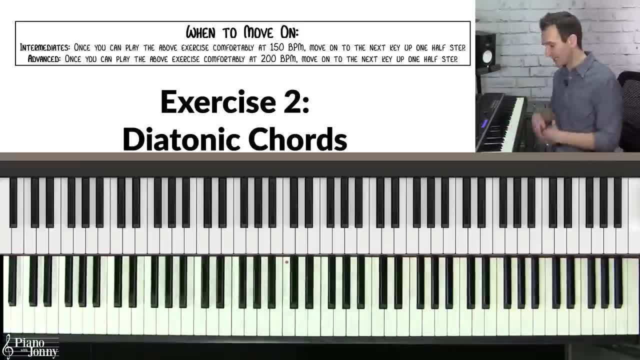 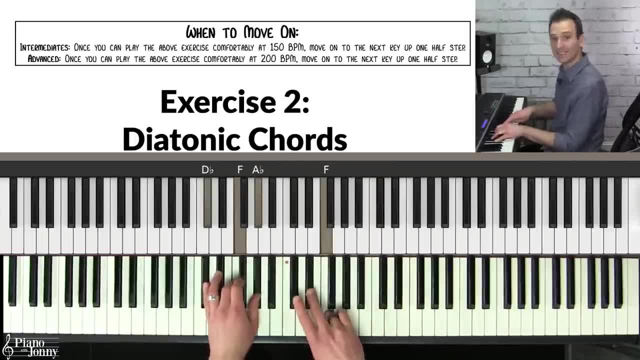 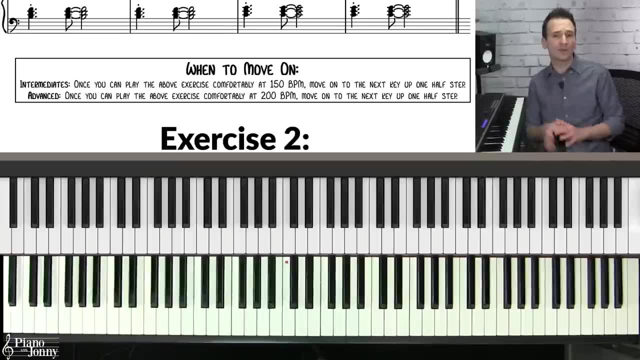 then I recommend that you do this exact same exercise in the key of D flat major, So same thing, E flat minor, F minor and so on. By the way, if you want to learn how to solo with each of your modes, 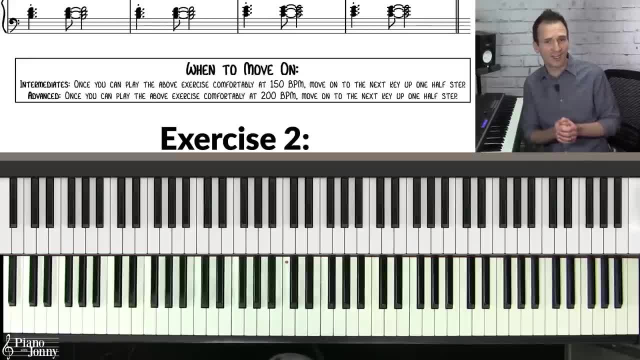 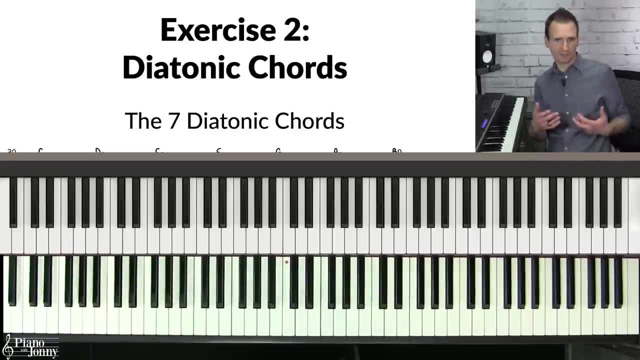 you can learn in our Soloing Fundamentals Learning Track. I'll put a link to that below. Exercise number two is to master your diatonic chords, and diatonic chords are simply the chords that come from a key. So if you're playing jazz tunes, 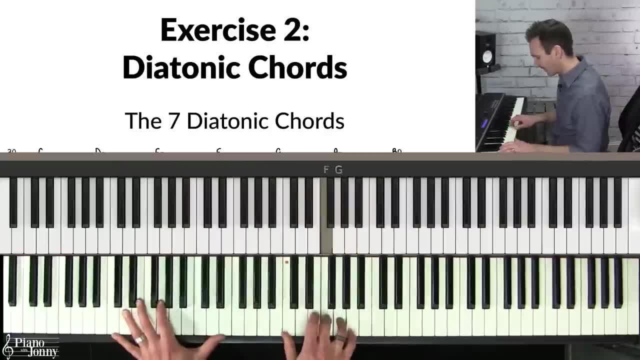 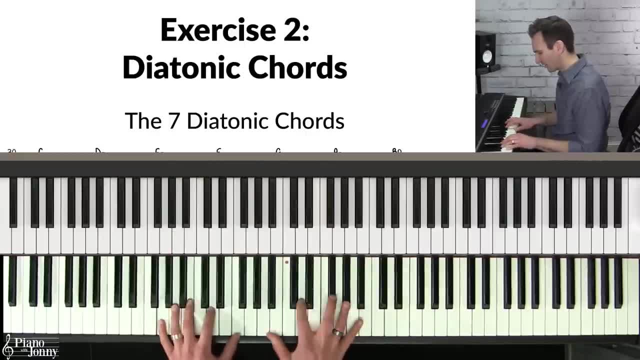 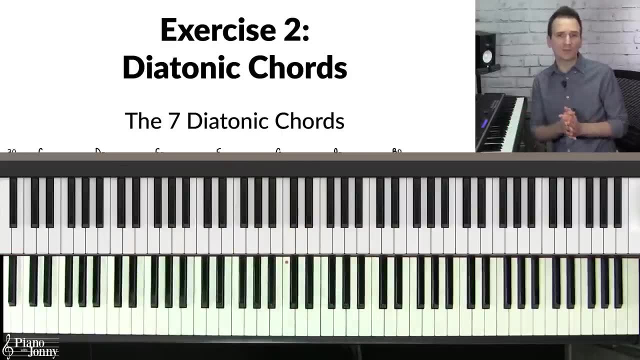 like Fly Me to the Moon. guess what? All of these chords come from the key of C major, or Autumn Leaves. All of these chords come from the key of G major. So you need to practice playing all of your diatonic chords. 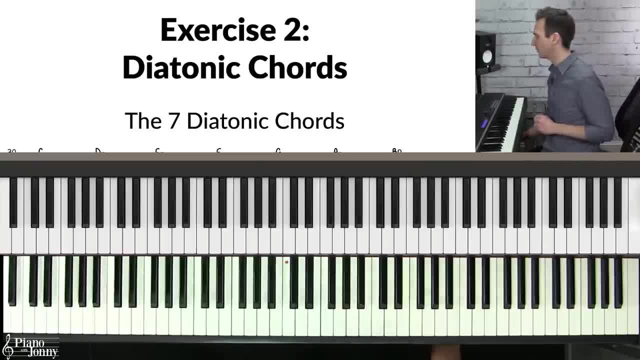 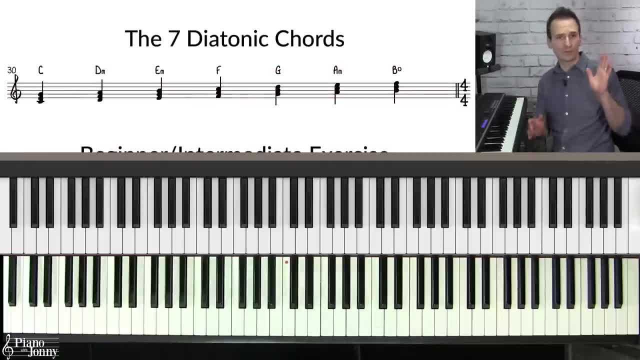 in all 12 keys to truly master jazz piano. So first I'm going to show you a beginner to intermediate level exercise, then an intermediate to advanced level exercise. So if you're more on the beginner to intermediate side, I recommend that you play your diatonic triads. 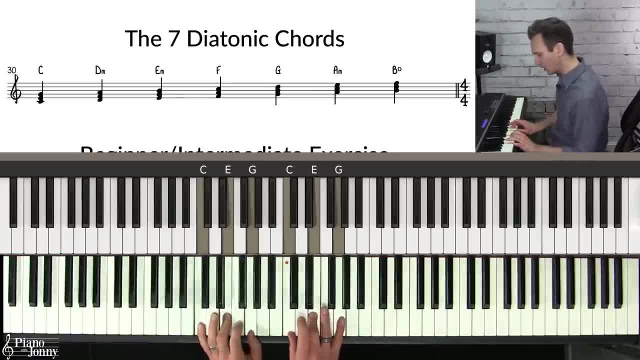 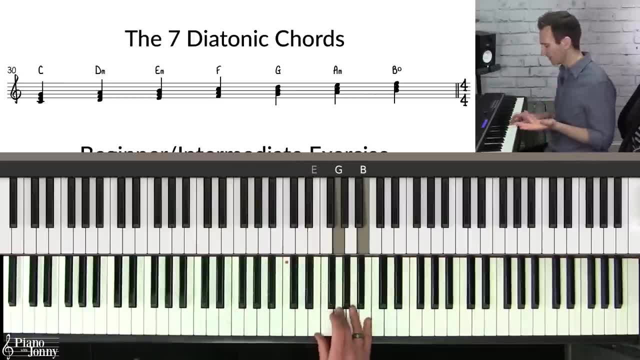 in a major key And basically these are all of the three note chords that come from the major scale. So we have C major, we have D minor, we have E minor, F major, G major, A minor and B diminished. 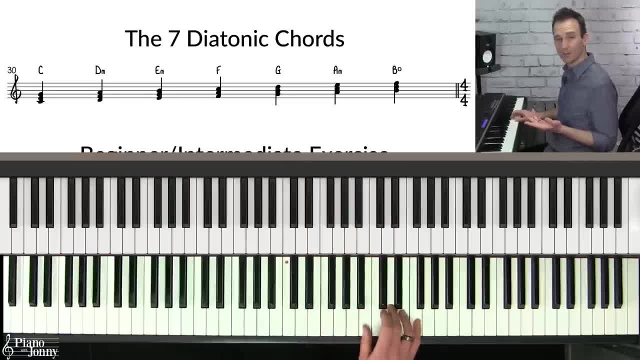 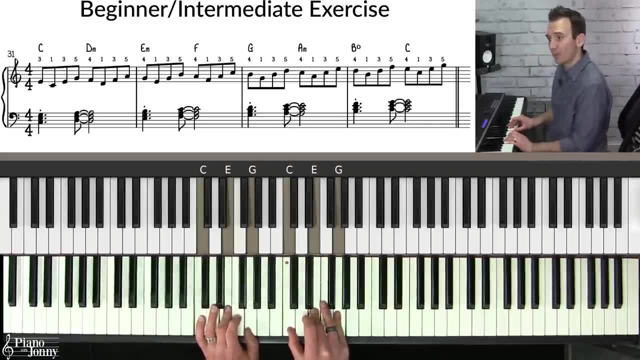 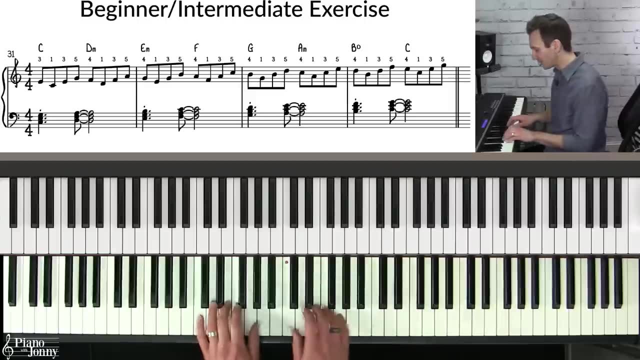 Okay, They're all of the three note chords that come from the major scale. So a very simple exercise is to take each of these chords and break them up using a simple pattern. Okay, Doesn't that sound nice? It's actually really simple. 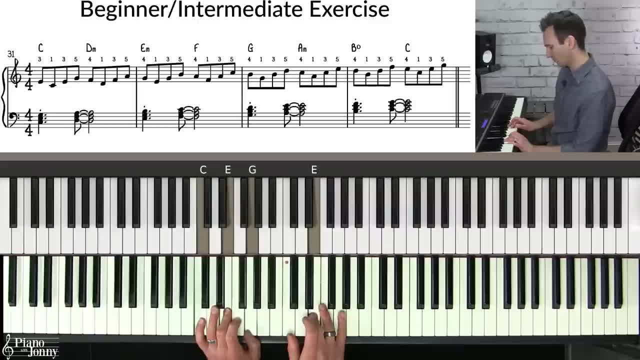 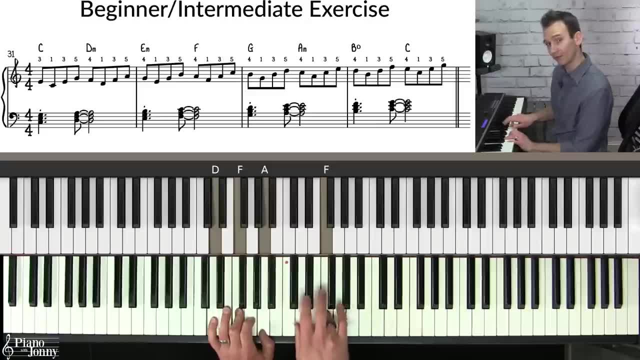 I'm basically taking each chord starting on the middle note, going middle bottom, middle top, And then on the next chord, D minor, I start on the middle note, but I use my forefinger. Okay, So middle. 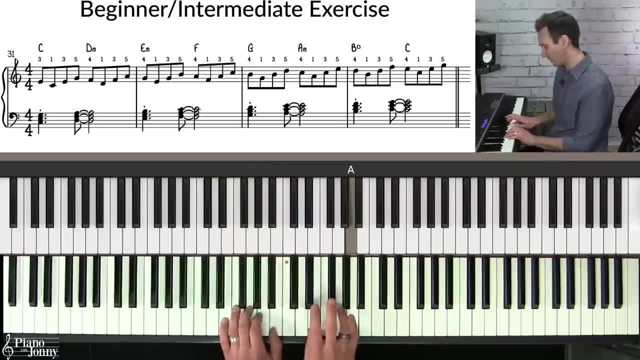 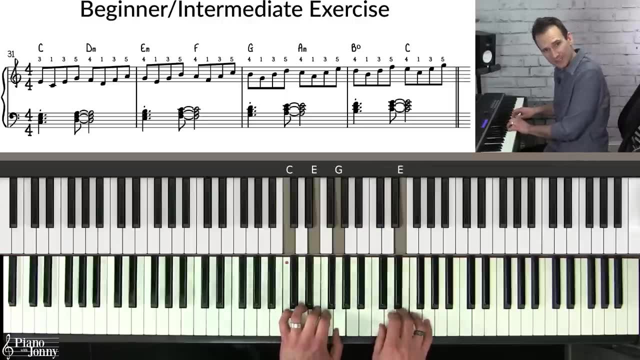 bottom, middle, use the third finger, top, And then E- minor middle, bottom, middle, top And then F- major middle, again raising the forefinger: the ring finger, bottom, middle, top, middle, bottom. 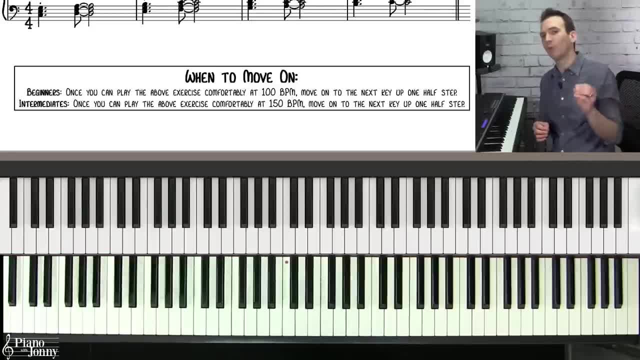 top. Now, if you're more on the beginner side, I recommend a target tempo of 100 BPM, And if you're more on the intermediate side, I recommend a target tempo of 150.. Now we have two backing tracks: a beginner and an intermediate one. 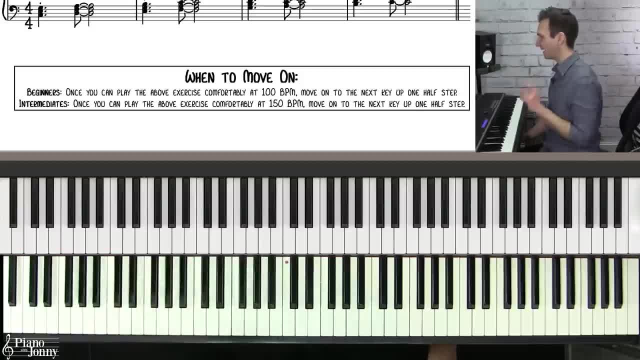 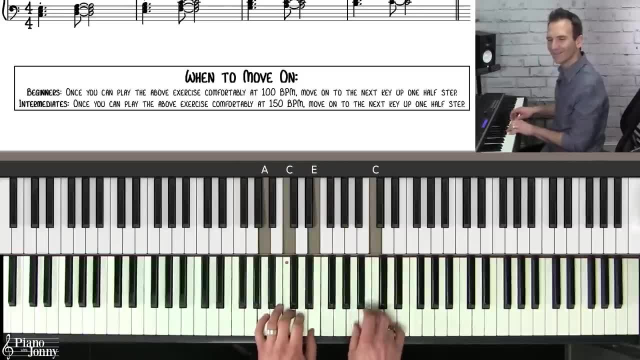 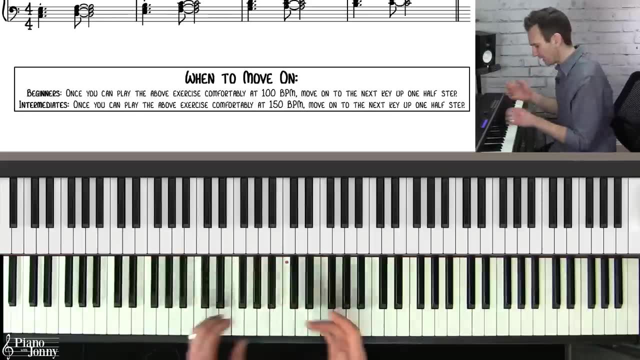 So let's go ahead and play this with the intermediate backing track, And here it is. Here we go Now. once you can play at your target tempo, then I recommend that you transition to the next key, next key, So you can play the same exercise in D-flat major. you need to know your diatonic chords. 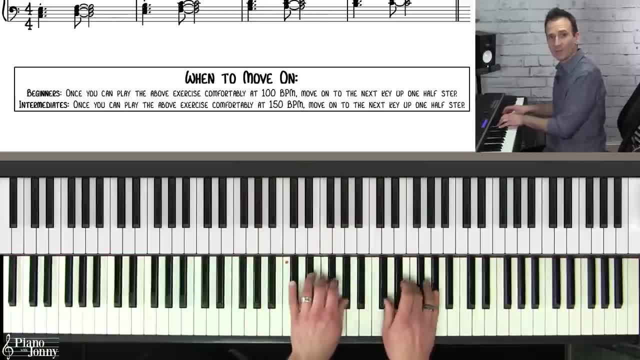 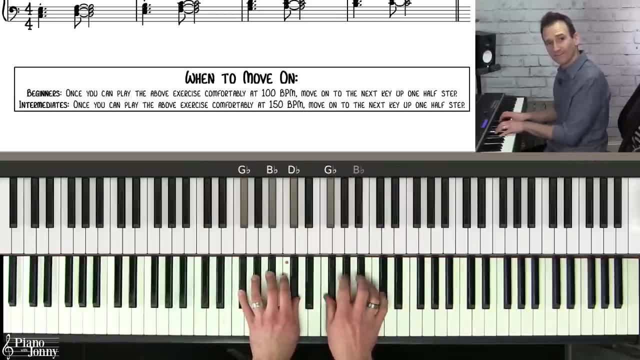 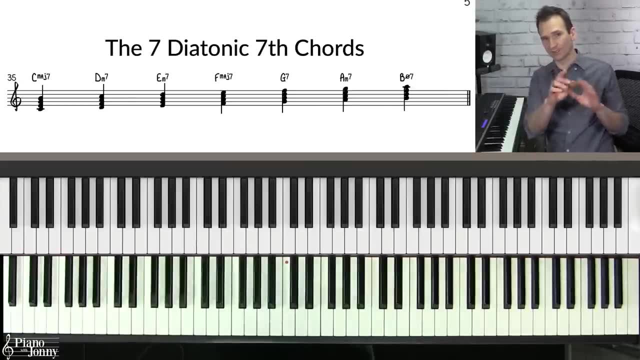 these are all of the three note chords that come from the D-flat major scale and then you can apply that little right hand pattern. Now, if you're more on the intermediate to advanced side, it's very important to learn all of your diatonic seventh chords in all 12 keys, and the difference between what I just taught you and the 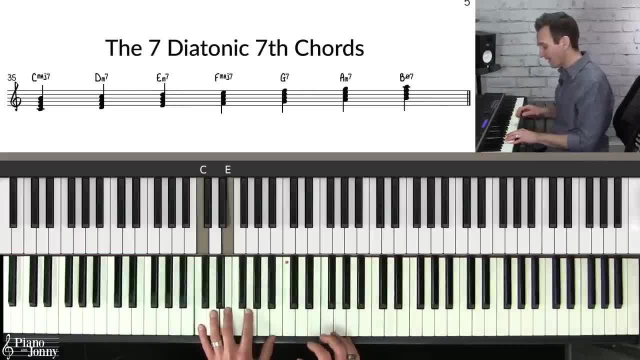 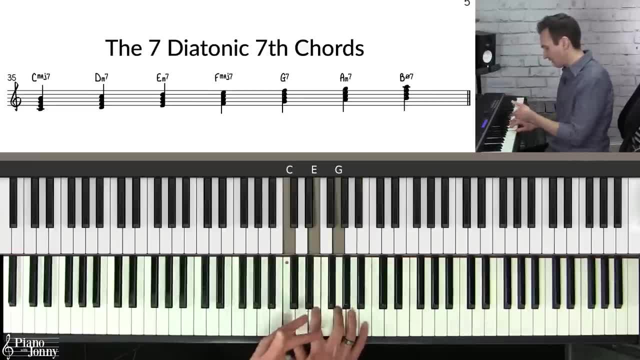 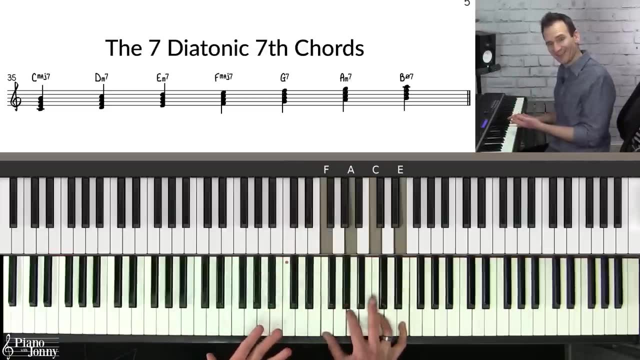 diatonic seventh chords is that you're going to add a seventh to each of the chords. So the first chord, C- major 7, we're adding another third on top of the C triad and then we do the same thing on the D minor. So D- minor 7, E- minor 7, F- major 7,- okay, G7, A minor 7, and B, half diminished 7.. 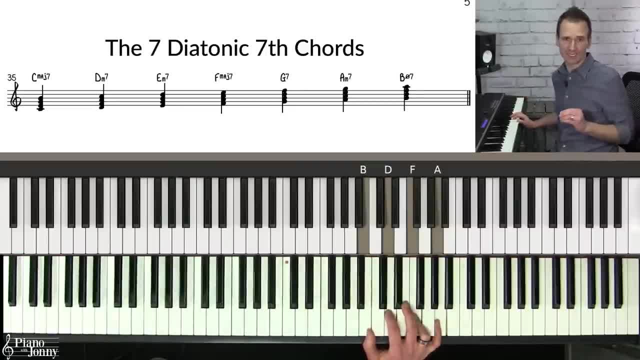 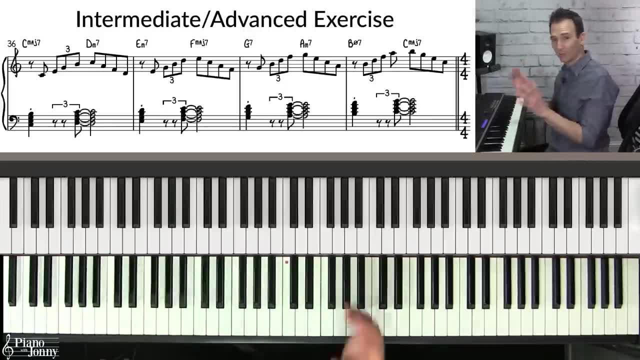 These are the most important chords that you need to know if you want to play jazz piano, All right. so here's the intermediate advanced exercise. Basically, you're going to take these diatonic seventh chords and you're going to do this sweet little pattern on them. 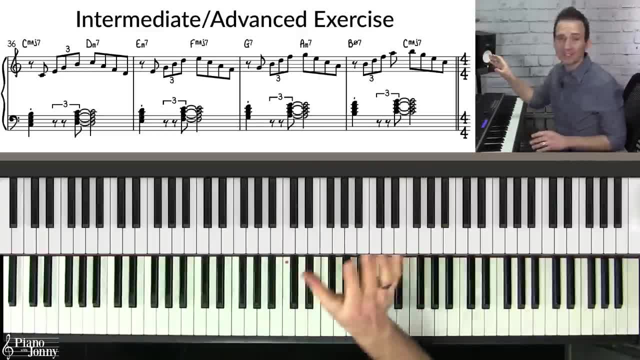 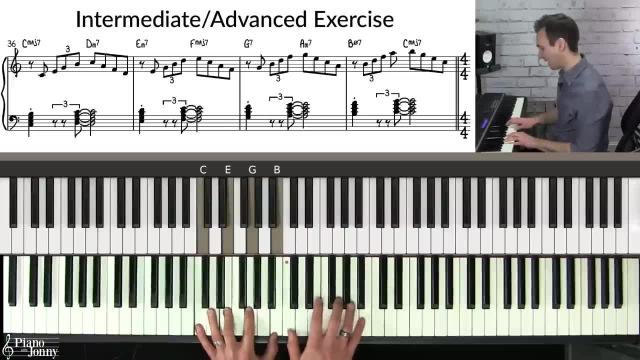 Okay, it sounds super cool and jazzy and I love this rhythm because it's so commonly used in jazz lines. So we're going to take our C major 7 chord, we're going to arpeggiate it up and then take D minor down. It's that simple. E minor. 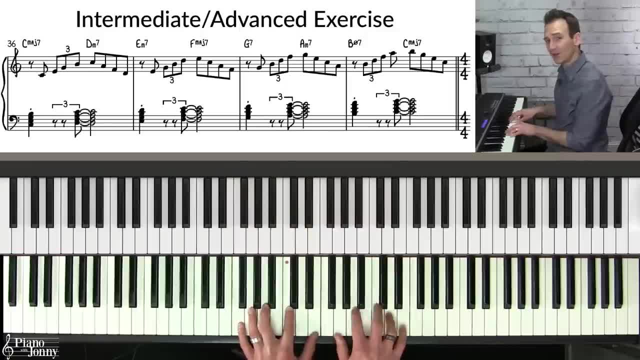 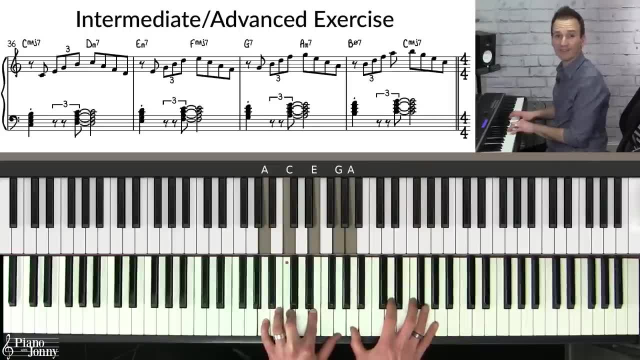 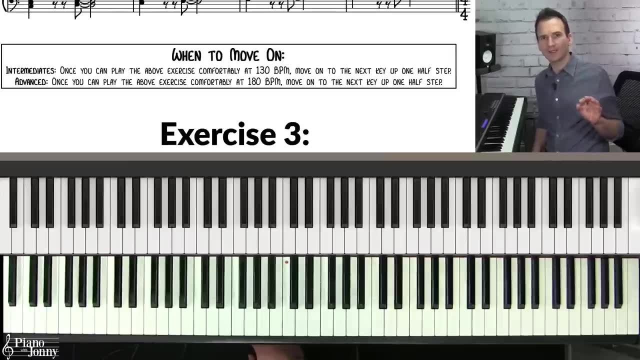 arpeggiate it up- F major down, G up, A minor down and B half diminished up and C major down. Now, if you're more on the intermediate side, a good target tempo is 130 bpm and if you're a. 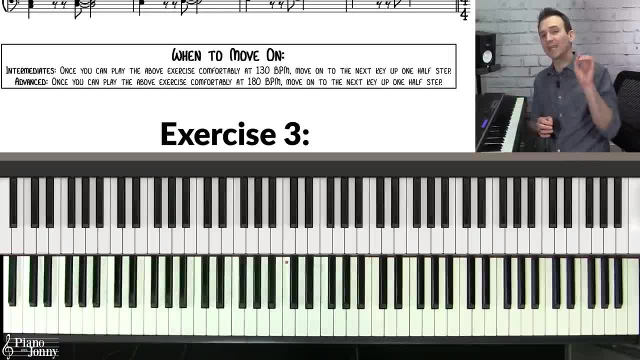 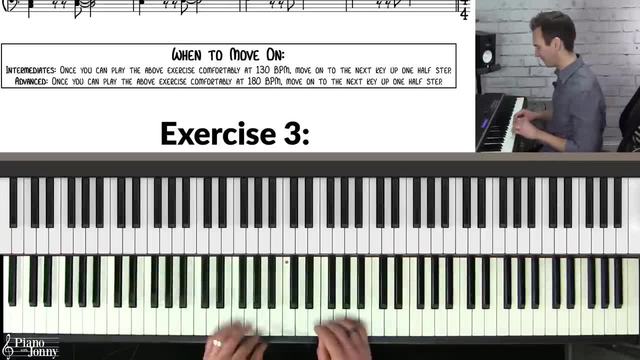 little more on the advanced side. a good target tempo is 180 bpm. So we're going to play this exercise with the intermediate backing chord. So we're going to play this exercise with the intermediate backing track at 130 bpm. Here we go. 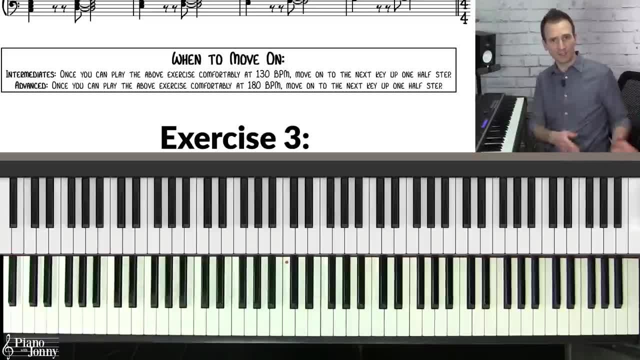 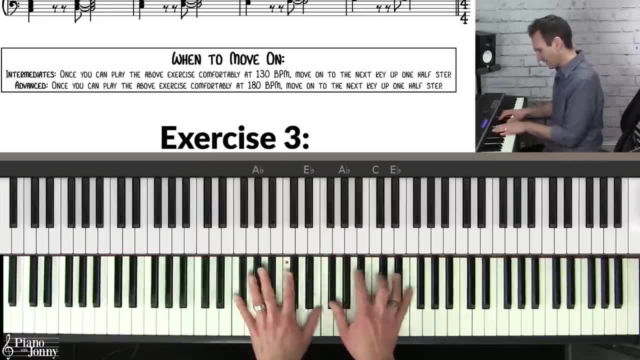 Now, once you've hit your target tempo, I do recommend that you practice this in the other 11 keys, So you could go to D flat major and practice all of your diatonic seventh chords that come from this key, and then you can apply this fun little pattern. 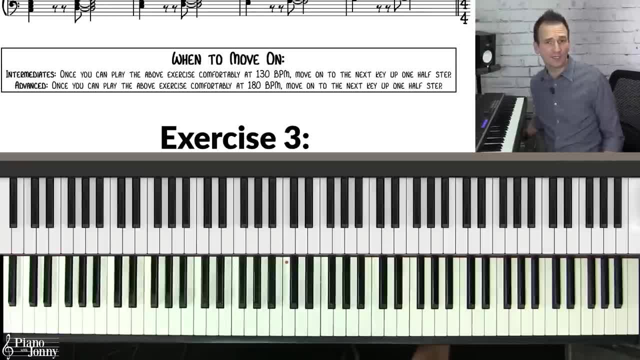 By the way, if you want to learn all of your diatonic seventh chords and all 12 keys, plus a bunch of amazing exercises to help you master them, check out our diatonic seventh chord exercises course. I'll put a link to that below. All right, exercise number three is probably 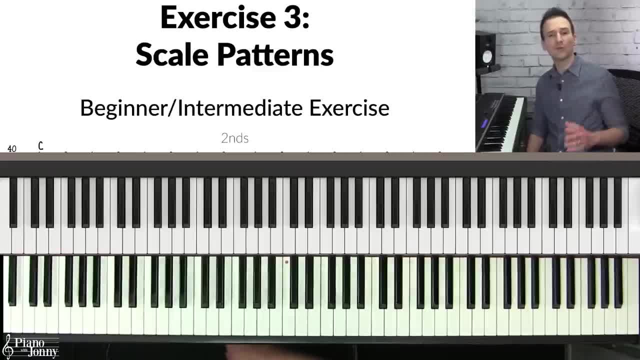 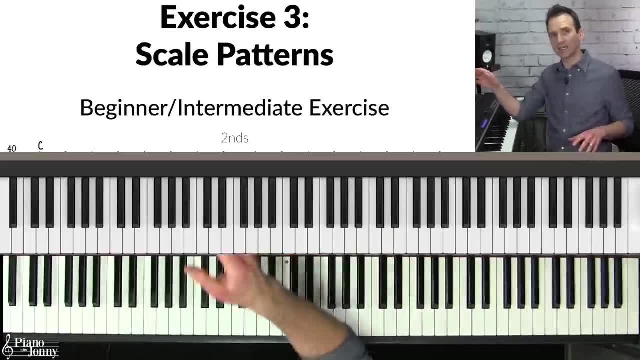 one of the most important exercises that you should learn if you want to solo on a jazz standard, And I'm going to actually go ahead and play a little solo to show you how this exercise will help you become a better soloist. I'm going to go ahead and play a little solo to show you how this exercise will help you become a better soloist. 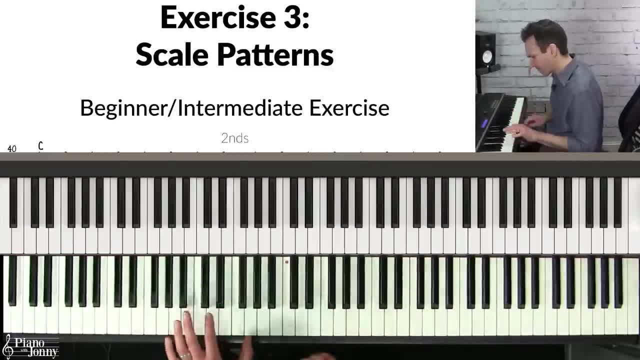 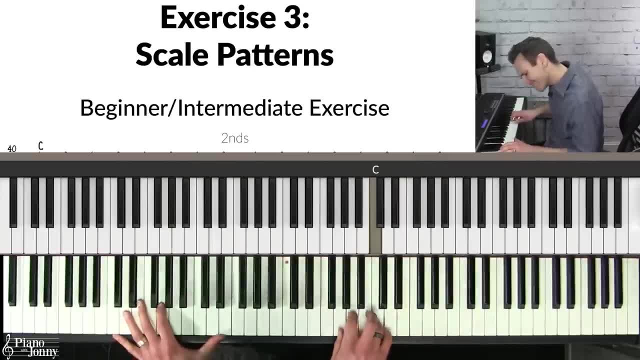 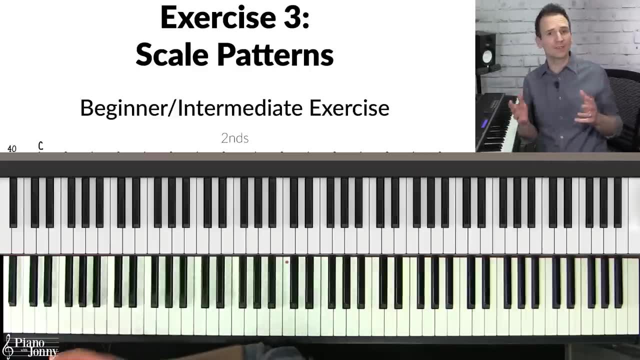 When I was just soloing, 99% of the notes that I played came from one scale, the major scale. But how was I able to create so many interesting lines using just one scale? Well, this exercise is what helped me to do it, and it's called the scale pattern exercise. I'm going. 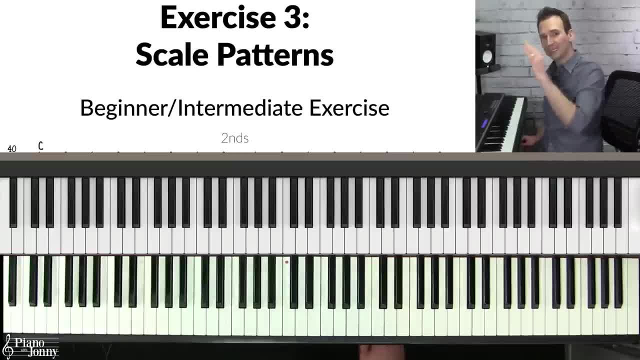 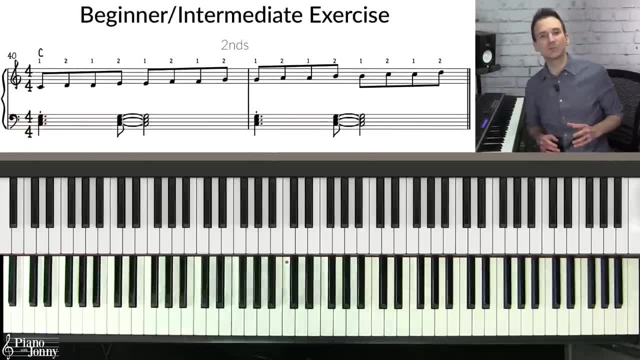 to show you an exercise for beginner to intermediate level players and then intermediate to advanced level players. All right, if you're more in the beginner to intermediate level. what you want to practice with this exercise is playing every interval using the major scale And. 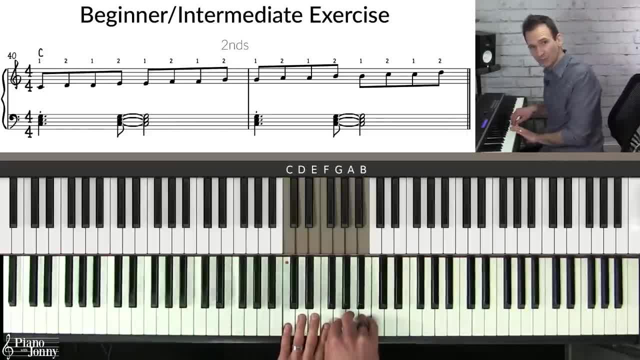 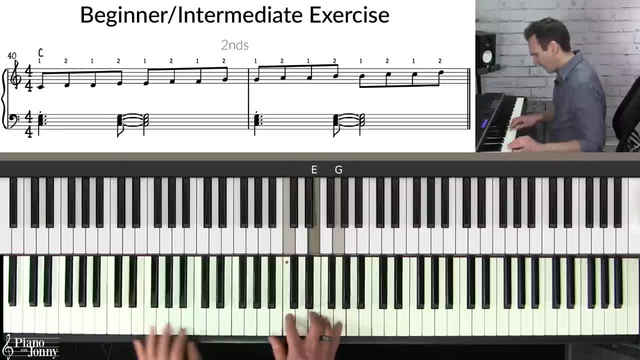 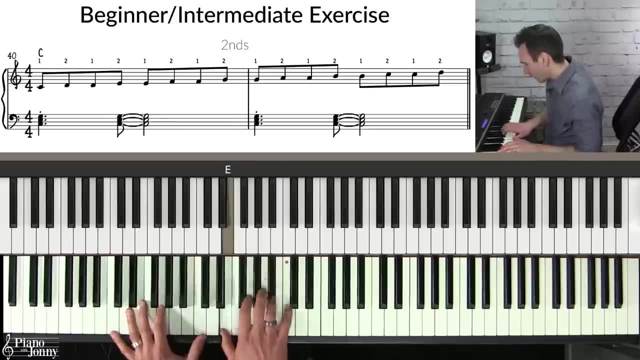 here's what I mean. If you only have seven notes to choose from, you really need to be creative with the types of intervals that you play Right? Notice, when I'm playing little lines, I'm being very creative with the intervals, meaning the distance between all of the notes. 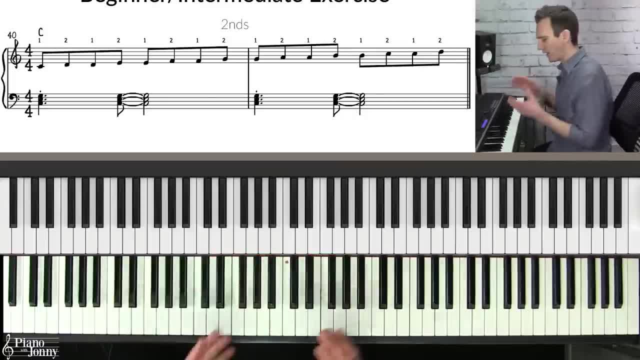 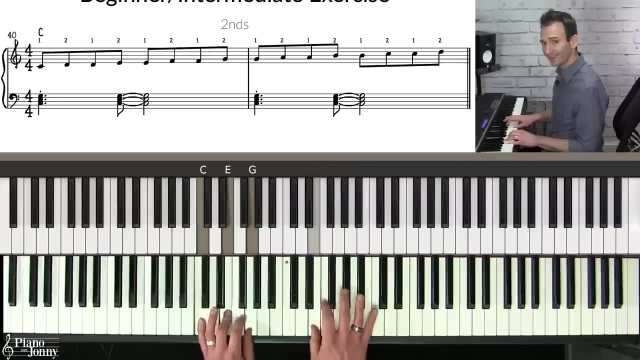 And so the way to practice intervals is to do this scale pattern exercise, And the way it works is we're going to first do our second interval, which is this, and we're going to practice this up the C major scale. Okay, It's actually really simple. So we go C, D, D, E, E, F, F, G, G, A. 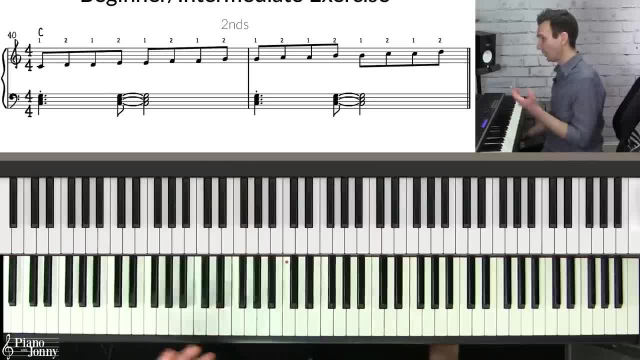 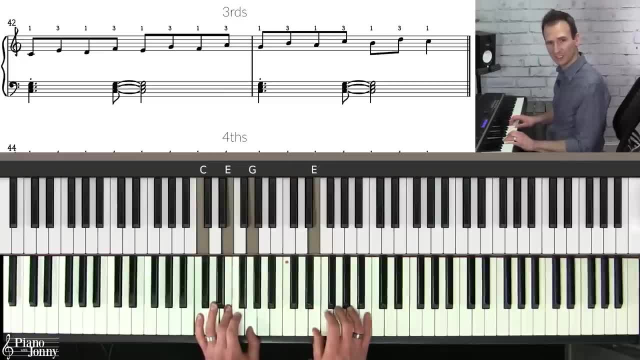 A, B, B, C. Okay, That's it. Once you've done that, then you're going to play your third intervals. So we play like this: C, E, D, F, E, G. See what we're doing. 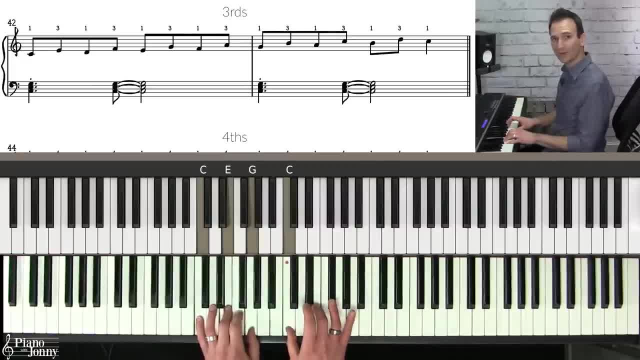 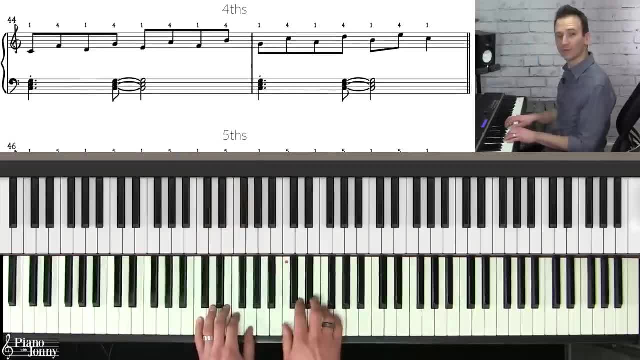 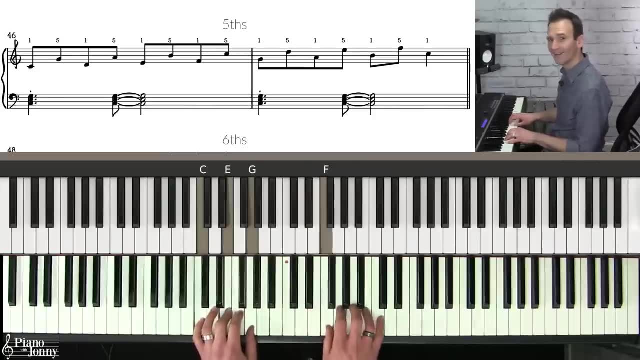 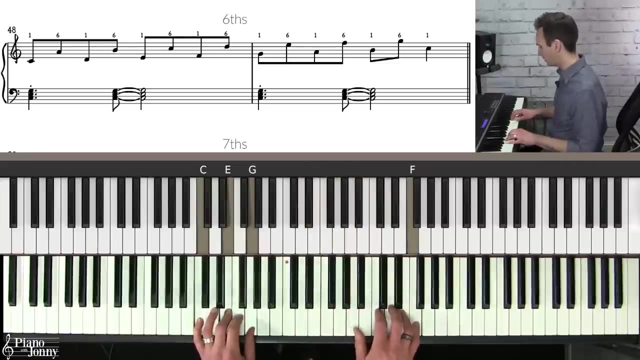 All the way up the piano, Okay, And it's really helpful to swing it Okay, It gives it a nice sound. Okay, Once you've done thirds, then you're going to do fourth intervals And then fifth intervals And then sixth intervals- Okay, And then finally, once you finish sixth, 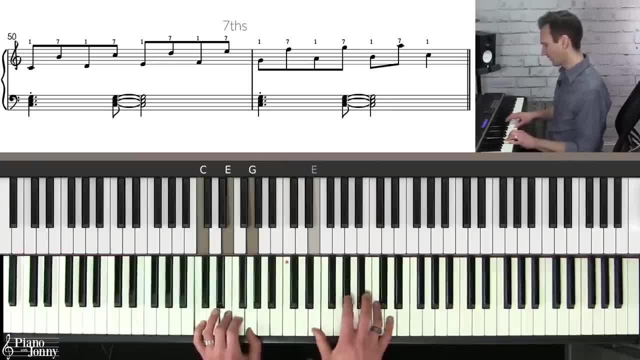 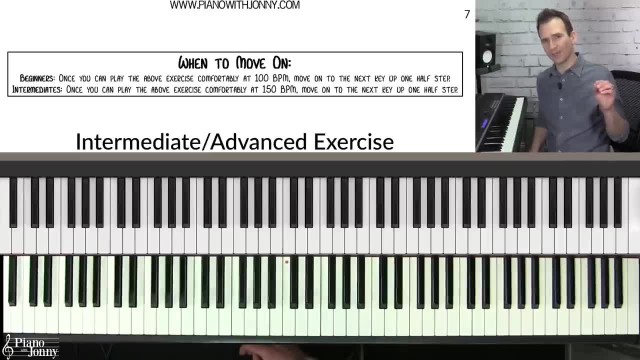 then you want to do your seventh intervals, And again I'm swinging it to give it kind of a lilting sound. Now if you're on the beginner side, you want to get this to 100 BPM, And if you're more on the intermediate side, you're going to want to do it a little faster. So 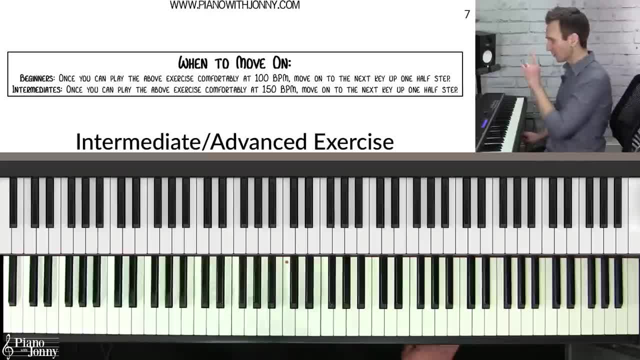 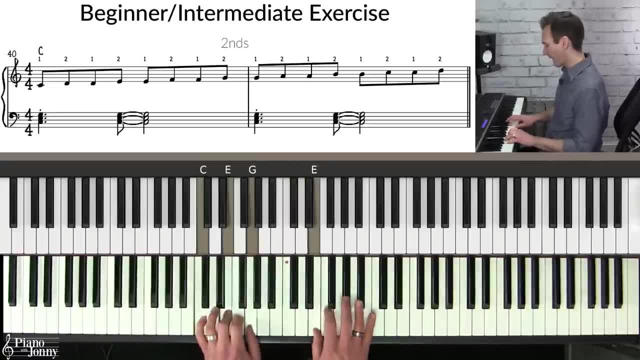 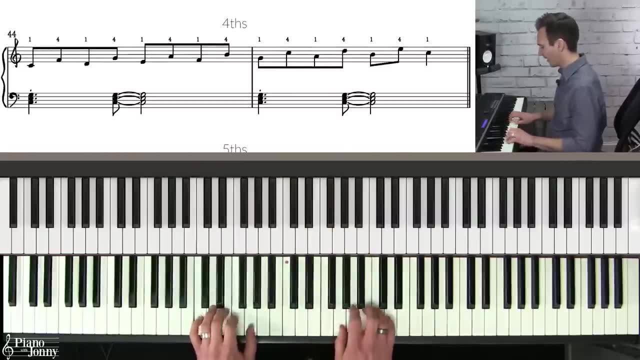 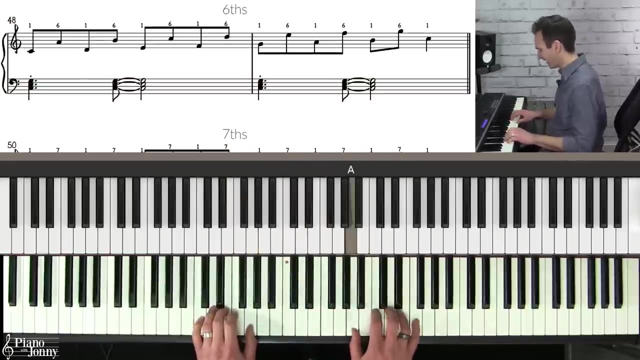 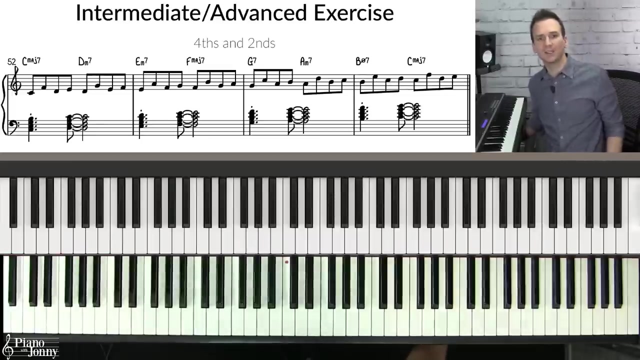 side, you want to get this to 150 bpm. So let's go ahead and play this with the intermediate backing track at 150 bpm. Let's start with seconds, thirds, fourths, fifths, sixths, sevenths. Now, if you're on the intermediate to advanced side, you want to practice your 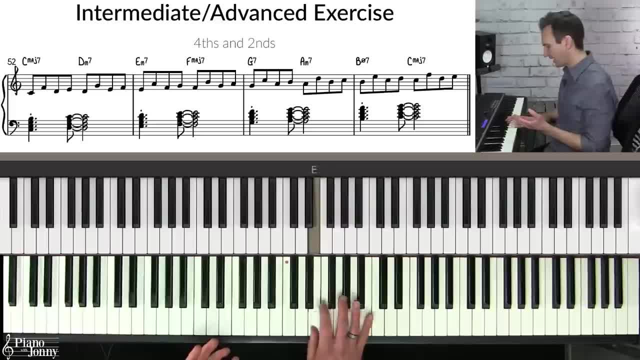 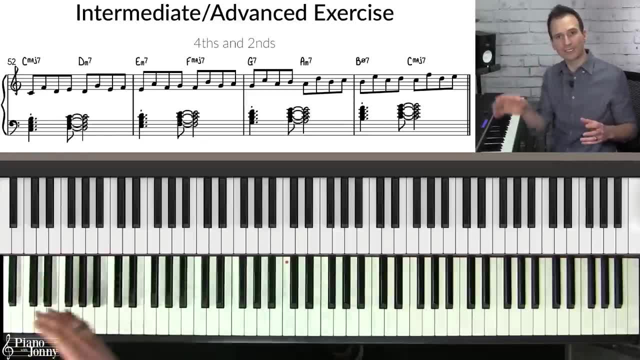 intervals. but instead of playing each interval by itself, you want to mix your intervals, because this is what pro jazz improvisers will do: They'll mix their various intervals to create some very interesting sounding lines. So there are three ways to do this. What I recommend: 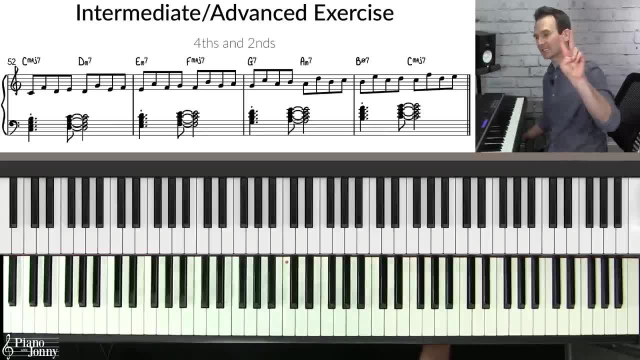 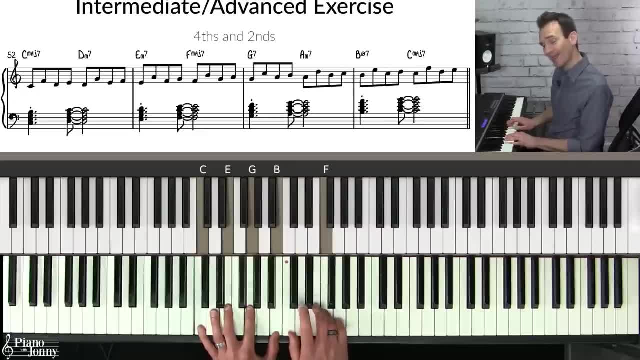 first is to play a combination of fourth and second intervals. So we're going to start on our C major, minor seven, and we're going to play a fourth interval, C, F, and then a second interval from the D, So D, E. That's our pattern. Then we're going to repeat the same pattern, except this. 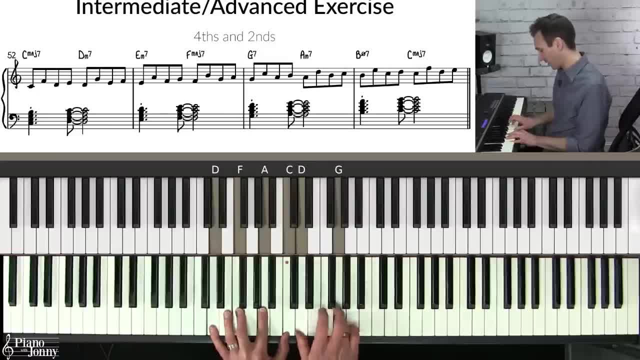 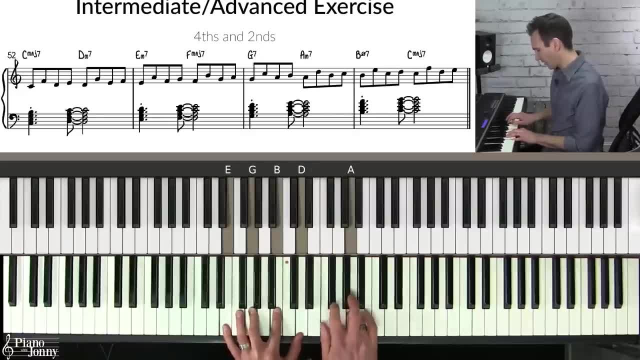 time. we're going to do it on the D minor seven. So up a fourth, and then we're going to do a second starting from the E. You see that- And then up to the E, Up a fourth. we're going to go down a third and then up a second. Does that make sense? Are you seeing the pattern? 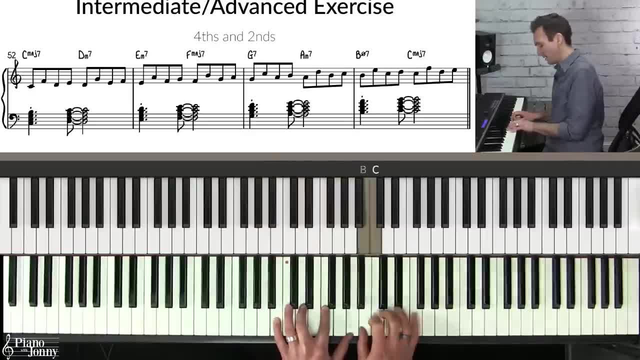 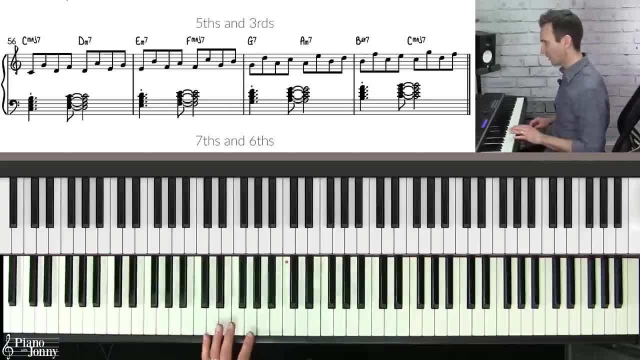 G, A, B, And then you can end on your C. Alright, next you want to mix your fifth interval with your third interval. So for this exercise, we're going to start on the C, go up a fifth and then we're going to do a third from the. 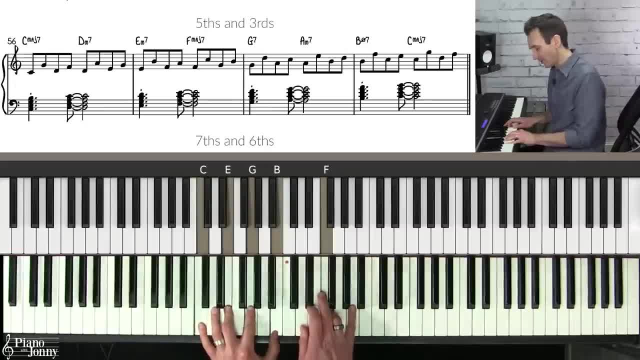 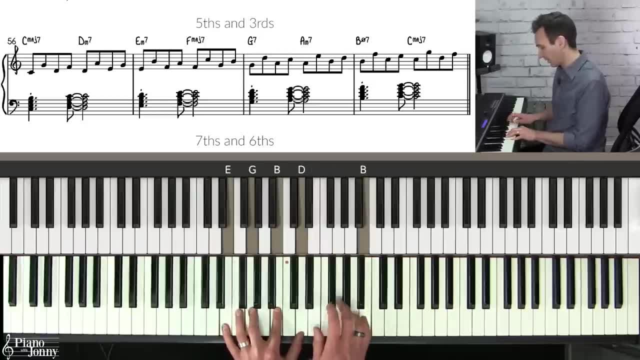 D, So D to F, And then we're going to repeat this pattern on the D, So up a fifth and then a third from the E, And then on the E we're going to do a fifth and then a third from the F, And then the same thing on the F. 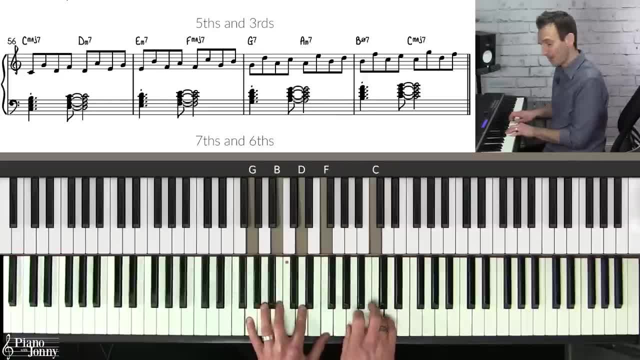 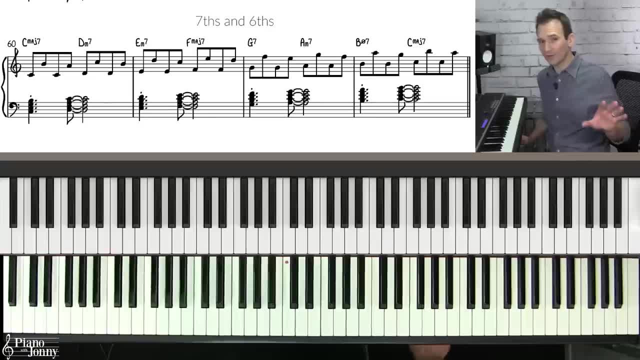 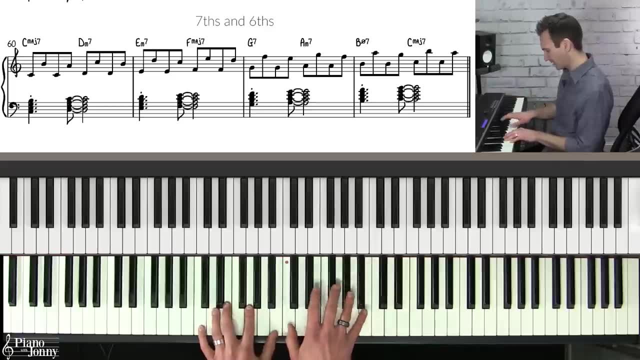 D, G, A, G, A, G, A, B, B, B, And then G, G, A, B, B, and then B, and then we can end on the C. Alright, we've covered all of our intervals except a seventh and a sixth interval. So for the final exercise we're going to play a seventh interval from. 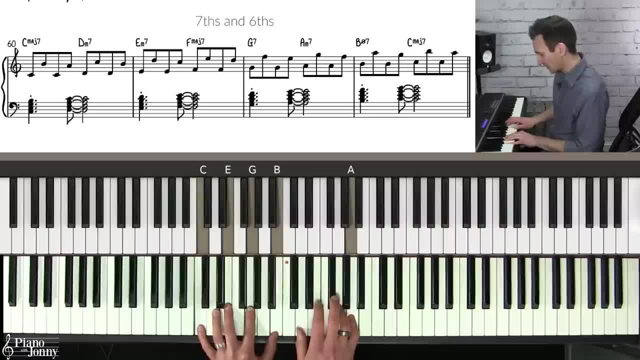 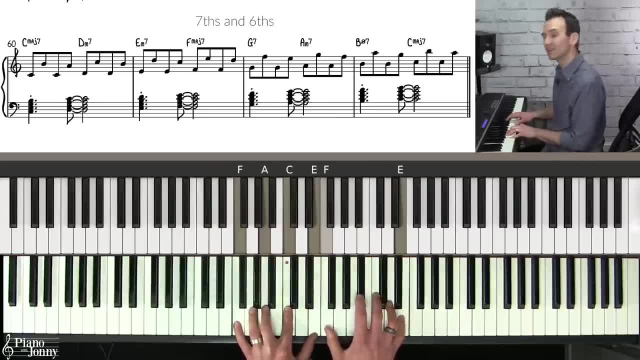 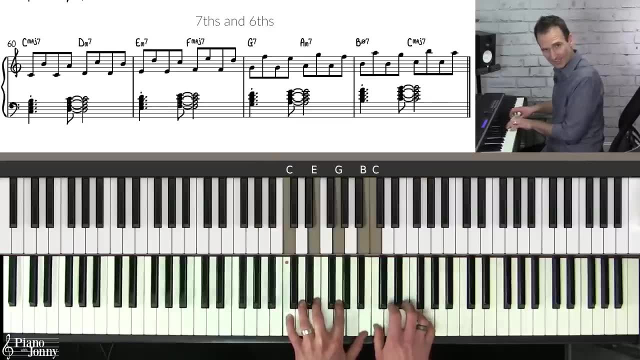 the C, And then we're going to play a sixth interval from the C, Make sense. And then same thing on D: Seventh, Sixth, Seventh, Sixth, Seventh, Sixth, six, seventh, six, seventh, six, seven, six, and then we end on C. Now intermediate players.